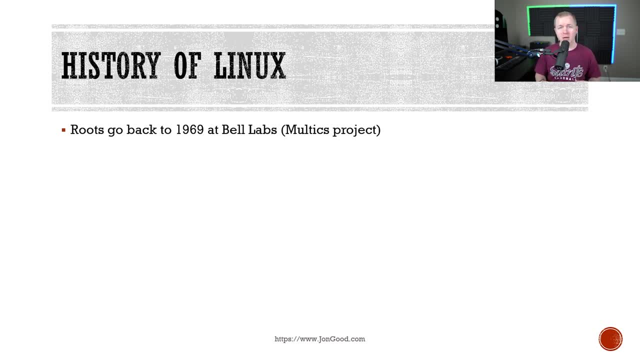 called the Multics Project. It was a Unix project and they were focusing on developing the Unix operating system. Then we have the Linux kernel that was developed by Linus Torvalds much later, And the kernel basically is how the operating system interacts with the hardware. That's what. 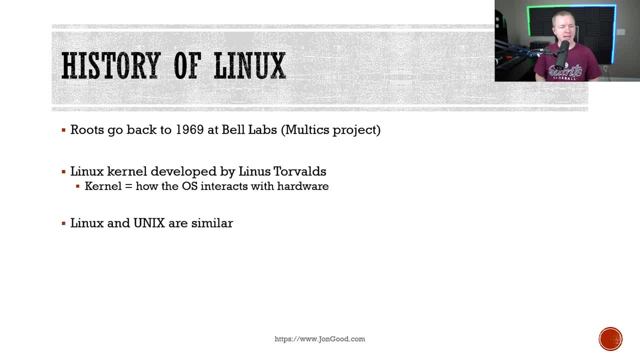 we mean when we say the kernel. Now, Linux and Unix are very similar to each other. They vary in some ways. Some commands are different, but they're very similar in the overall infrastructure. Unix is typically used for server functions. You're not going to find a lot of end users. 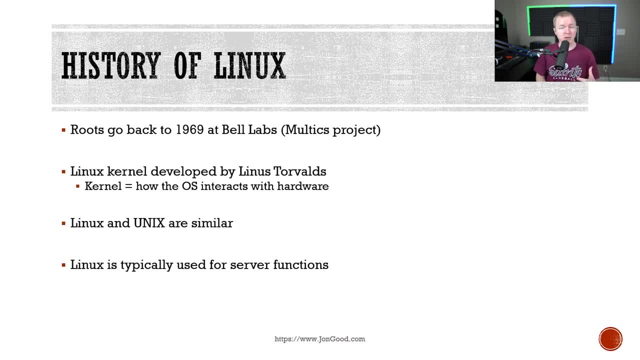 using the Linux operating system, although it's possible, and also computers like Apple are based on the Unix operating system, So very similar, And then operations vary depending on the flavor of Linux that you're using. We also call this the distribution, So unlike Windows, where you just have Windows 10 and Windows XP and Windows 7 and 9 and sort of what it is. we also call this the distribution. So, unlike Windows, where you just have Windows 10 and Windows XP and windows 7 and Windows 9 and Windows 10 and 7 and Windows eight and Windows ten and Windows maybe more than three times a DisParisan- 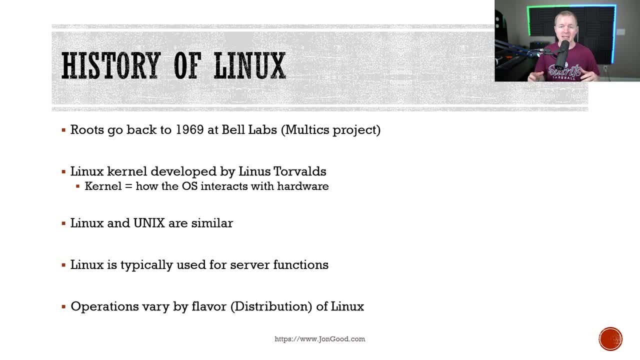 and there's just one flavor In Linux. we have Ubuntu, we have CentOS or CentOS and several different versions that you can be exposed to. So we're going to go into a demo now of installing Ubuntu. So in my lab machine here I'm using VMware Workstation Pro. 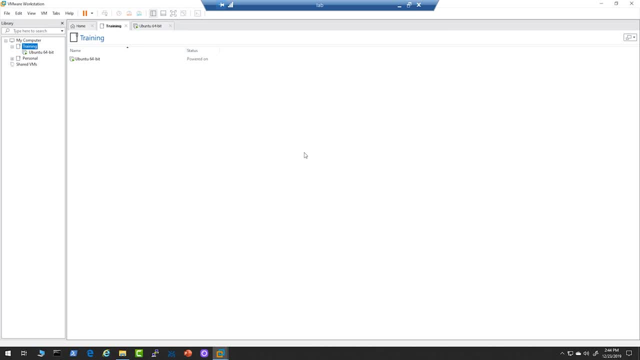 Now with virtual machines, there's some interesting intricacies. There are several different softwares that you can use for virtual machines. You have VirtualBox, which is free. You have Parallels on Mac. You have VMware Player and VMware Pro. 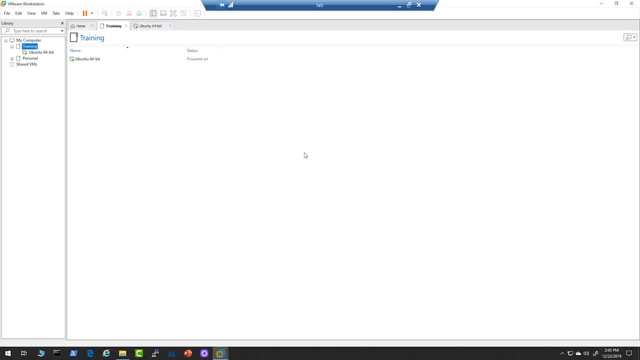 One thing that I've learned is VMware tends to be the most stable software for virtual machines. You also have Hyper-V with Microsoft, which works pretty well. Now, the reason why I recommend VMware is because a lot of VMs out there, and if you get a VM from somewhere else, 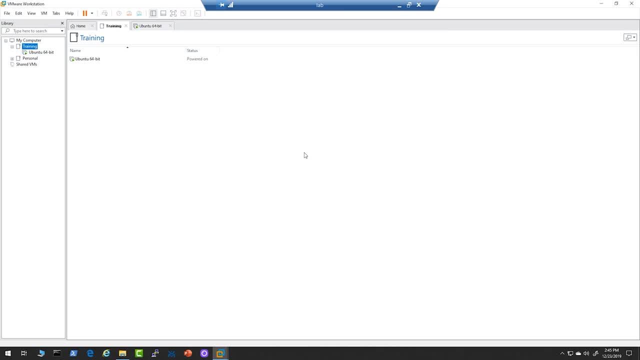 say somebody creates one for you or you're downloading a practice virtual machine, a lot of those will be built with VMware. I've run into issues personally trying to use VirtualBox and other instances where it just doesn't either work right or it won't even import the virtual machine. 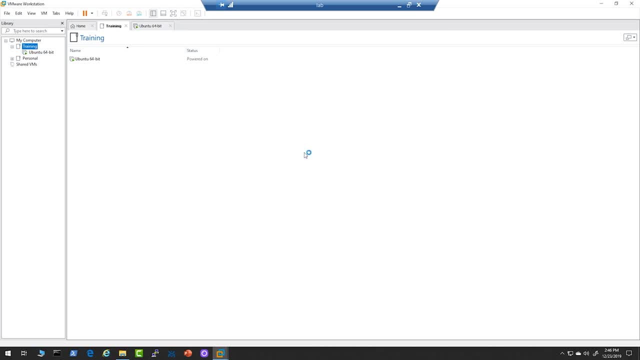 So I highly recommend that you use VMware Now. when you first go into VMware, when you're going to add a virtual machine, you would first go to the website and download the ISO file and then you would go to File New Virtual Machine. 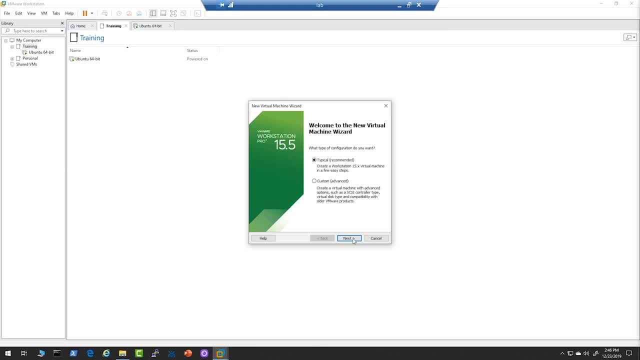 and then you're going to get this option. It would go Typical, and then you would browse to your ISO file. I've already created one, so at the end here I'm just going to exit out, But you put your ISO location in there. 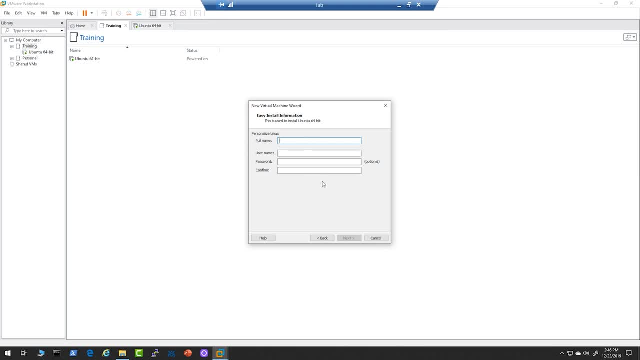 You would go through and you would type. you know whatever you're going to use. So create a basic username with a password and then you would put in your name of your virtual machine and where you want to store it. You pick how big you want the hard drive to be. 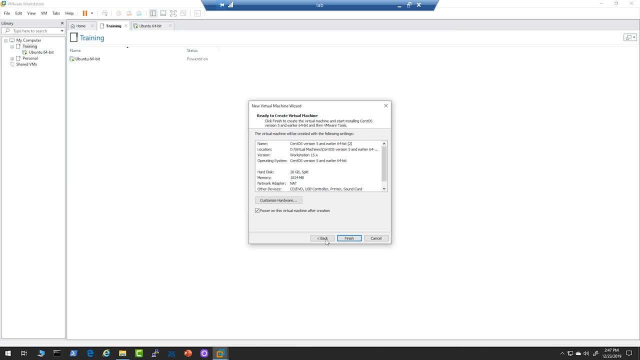 And again, I would just go through, and then I would say: go through and use the defaults, And then you can customize the hardware that you want to use as well, If you want to use more RAM or maybe make the hard drive bigger. 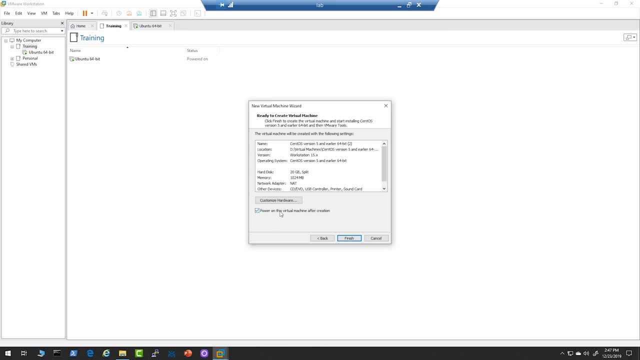 use more resources, like more processors, and then you leave this checkbox checked and then you hit Finish and then it's going to launch your virtual machine. Now I've already created one for Ubuntu, so I haven't hit any OK or dialog boxes or anything like that. 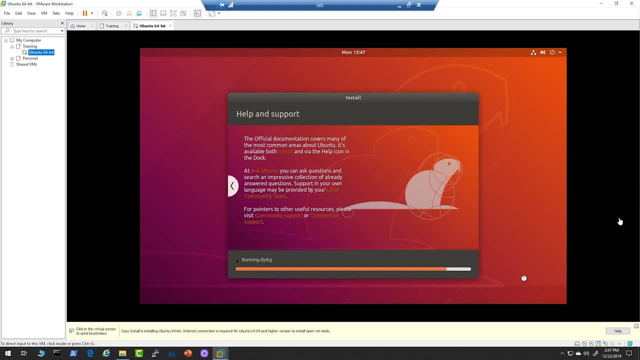 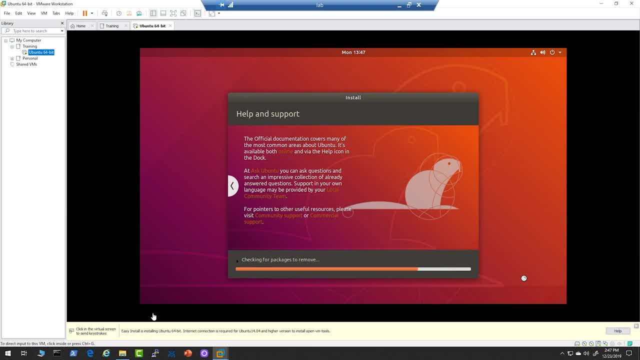 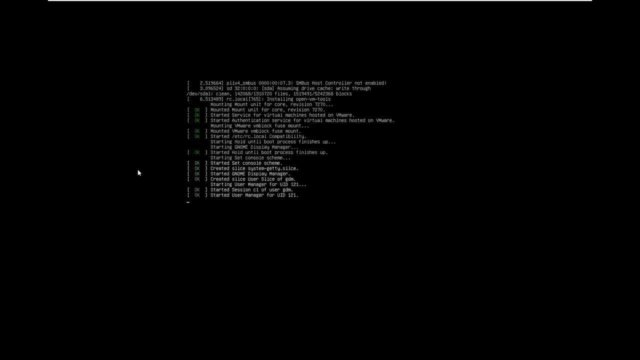 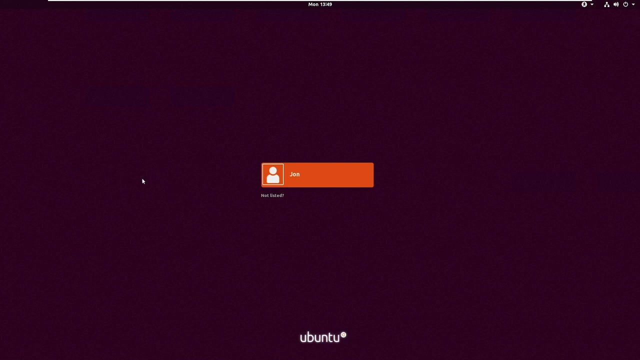 As soon as I hit the Finish it started into the screen, So it's preparing all the basic packages. The nice thing with VMware is that by doing that GUI, it actually creates a lot of the basic structure for you, So you don't have to do a lot of option selecting. 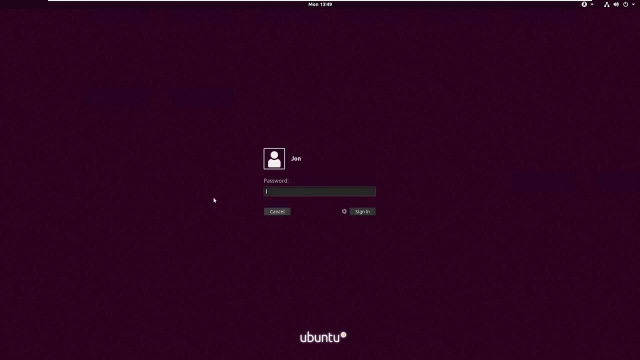 So now that it's set up, I can go ahead and click on my user here to log in. So now that it's set up, I can go ahead and click on my user here to log in. So now that it's set up, I can go ahead and click on my user here to log in. 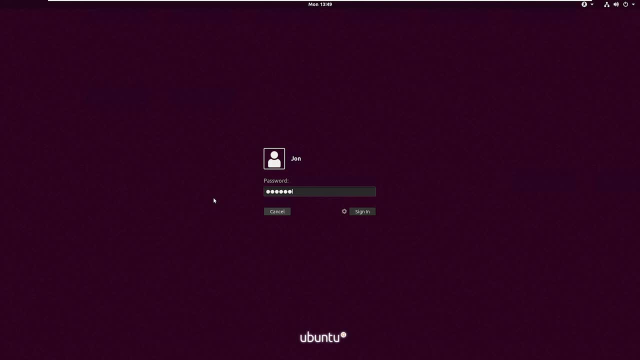 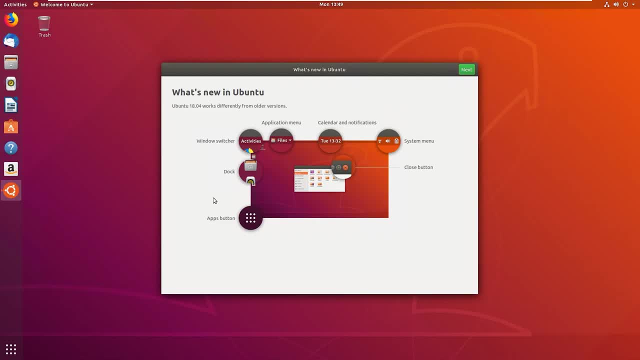 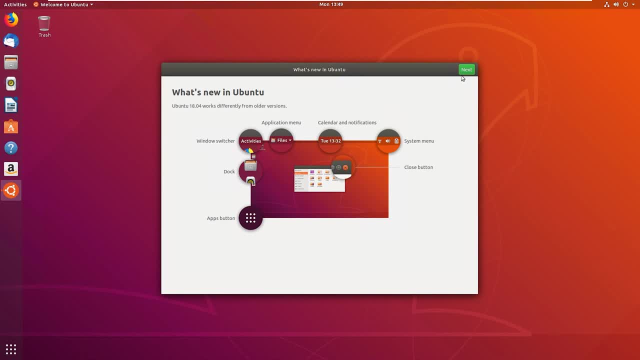 And now we are into the Ubuntu operating system, And now we are into the Ubuntu operating system, And now we are into the Ubuntu operating system. I'm just going to ignore a lot of this stuff. I'm just going to ignore a lot of this stuff. 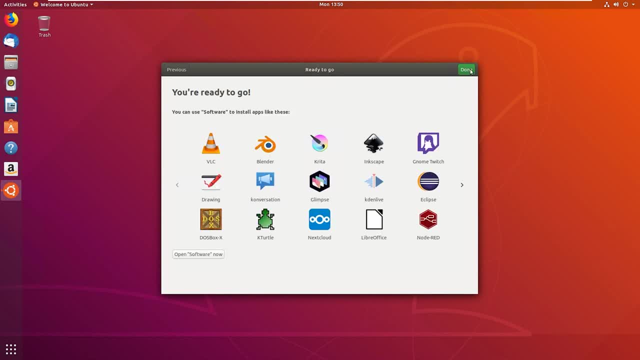 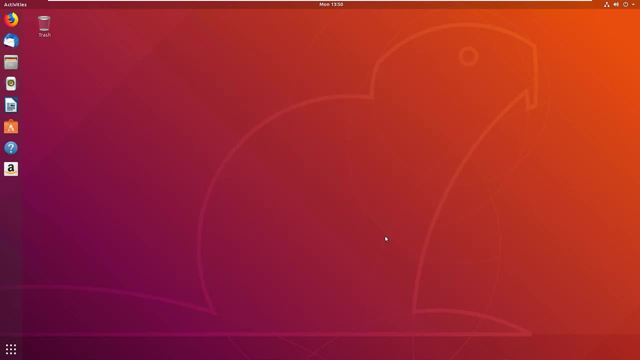 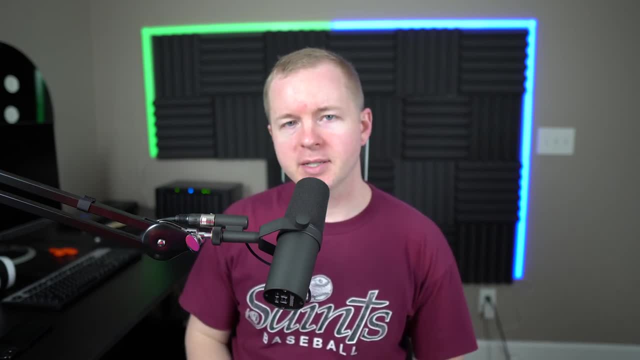 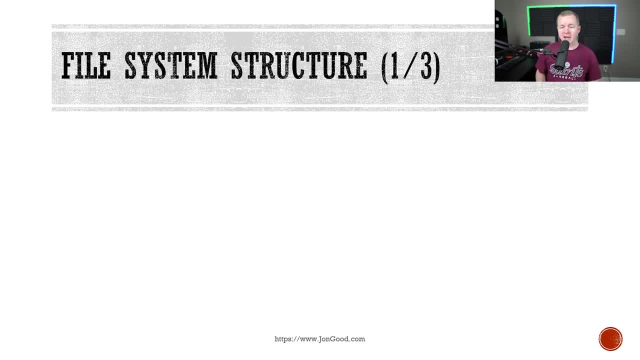 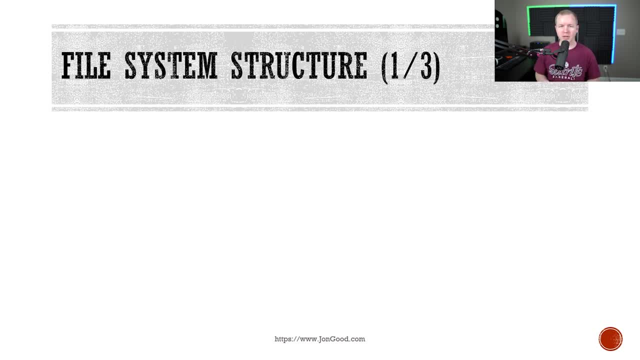 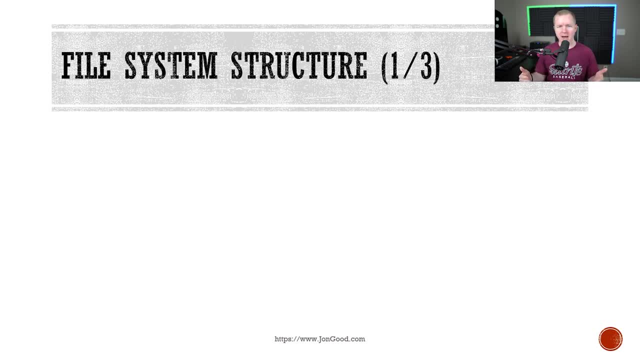 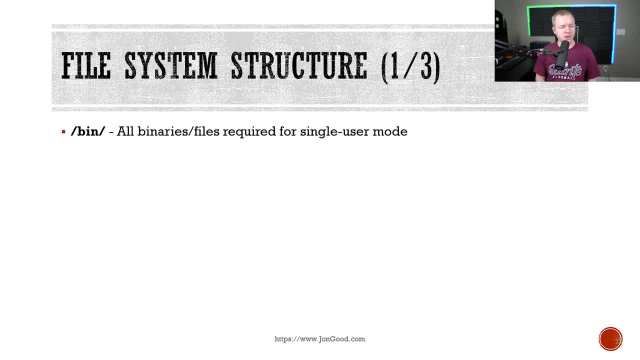 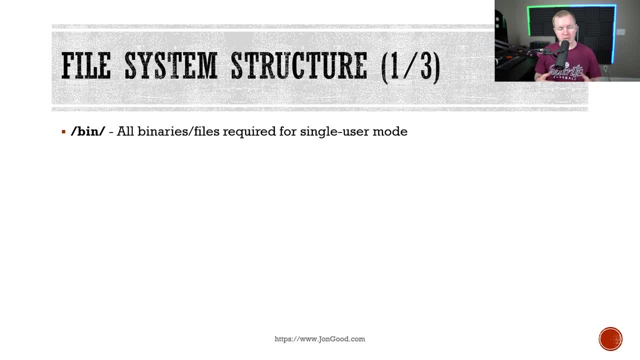 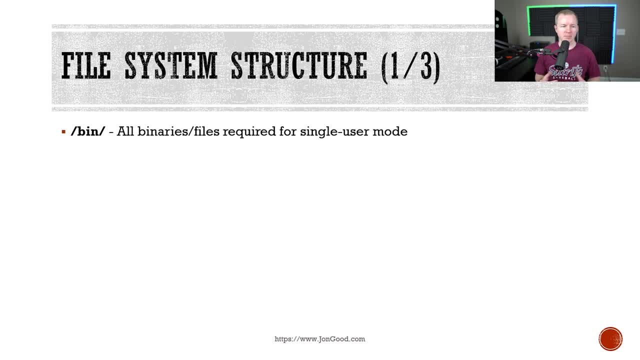 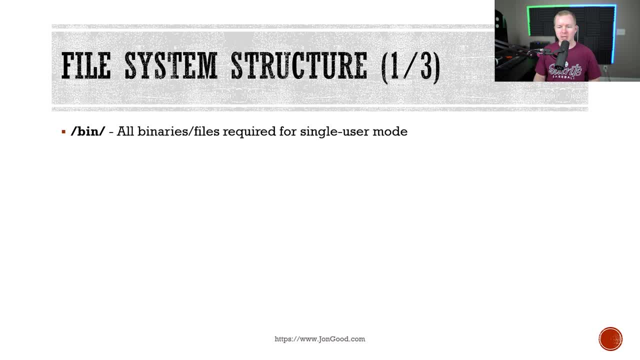 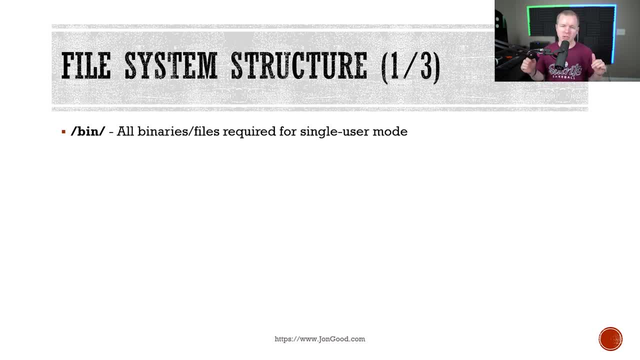 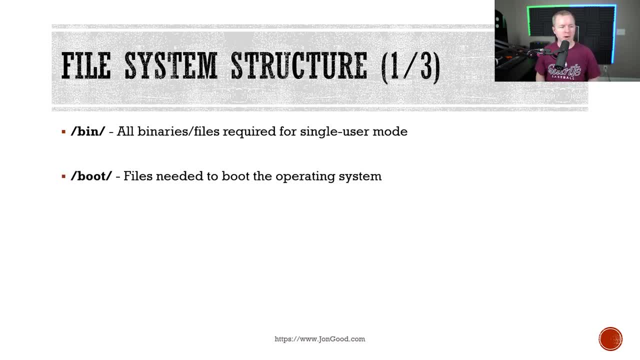 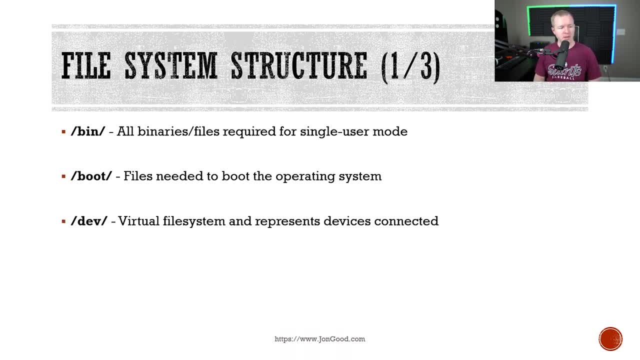 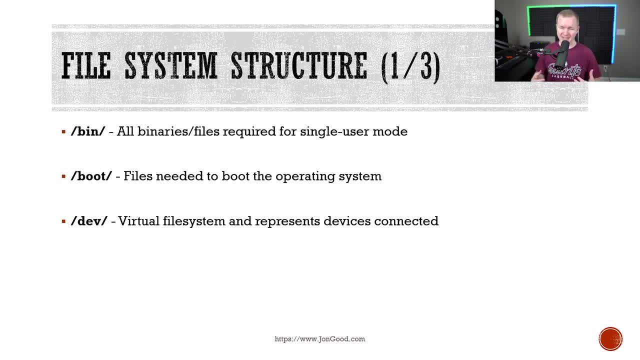 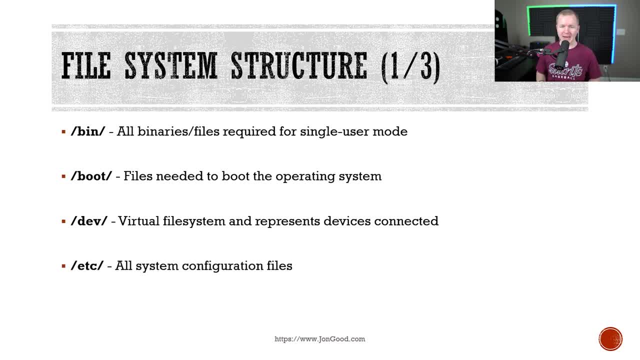 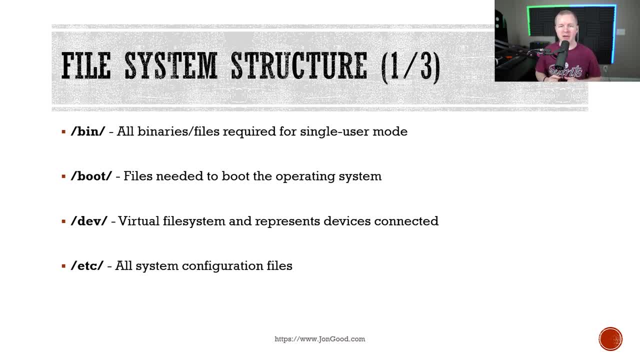 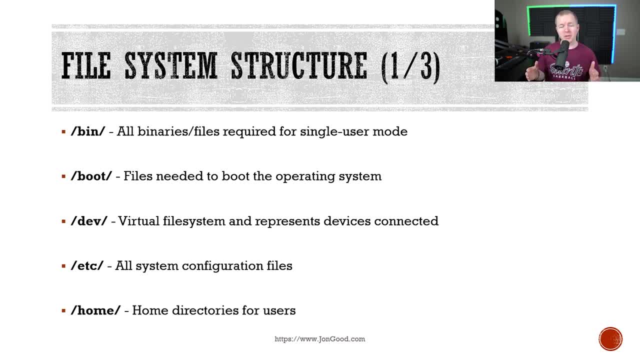 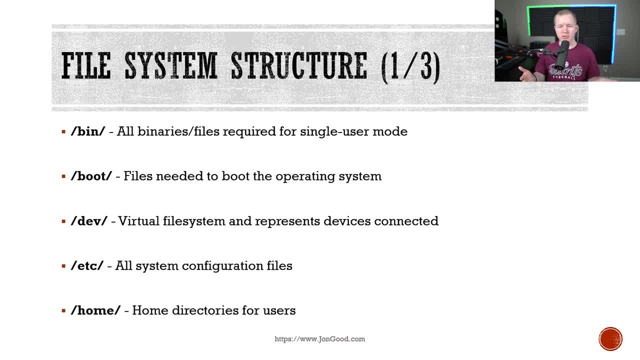 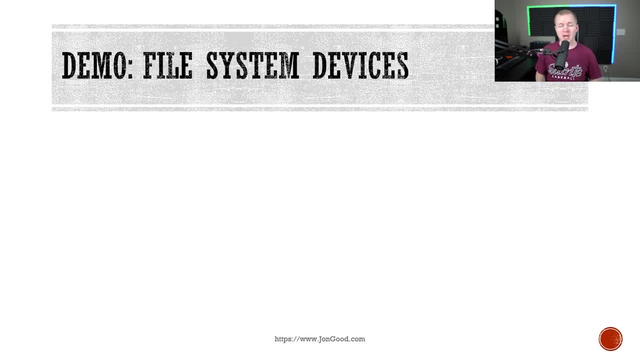 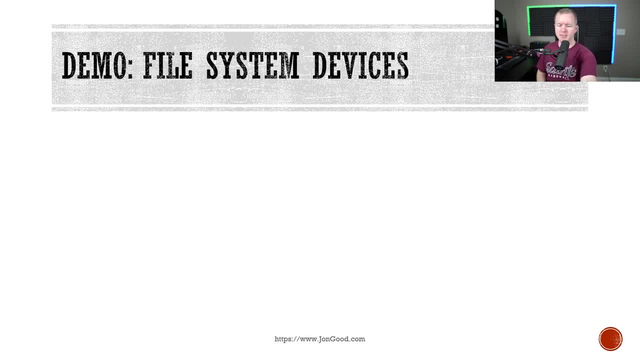 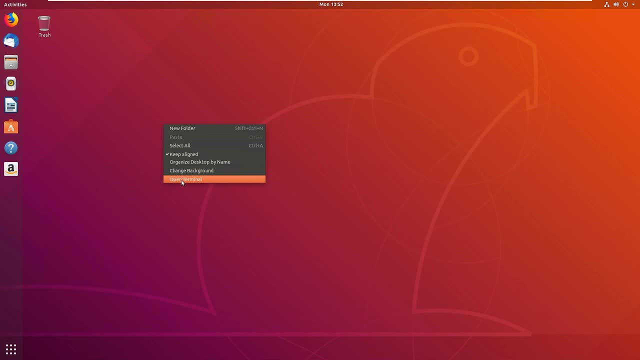 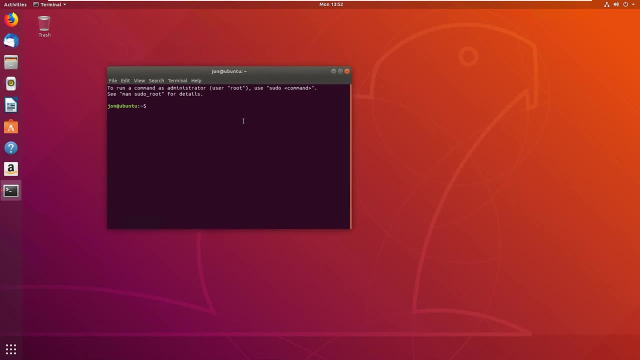 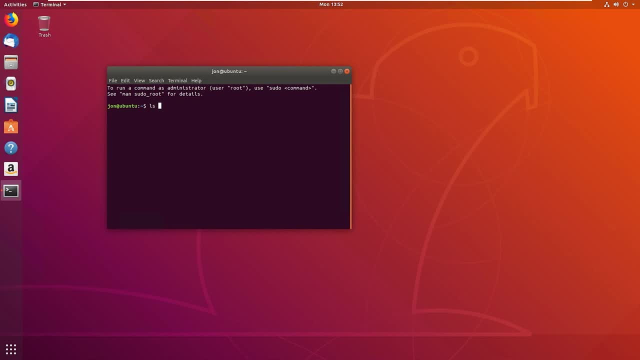 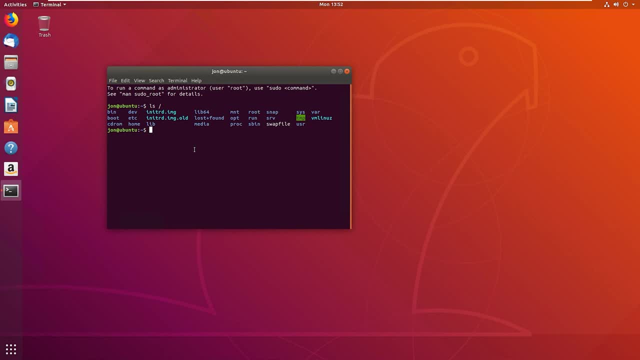 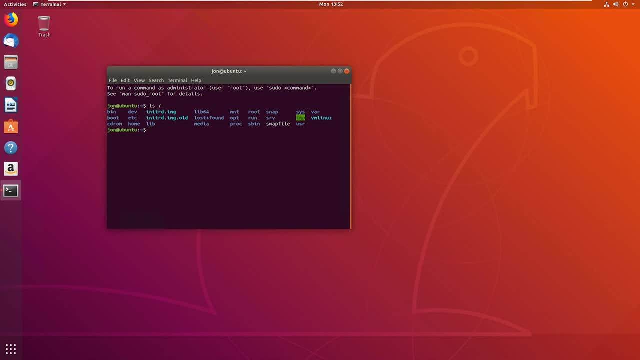 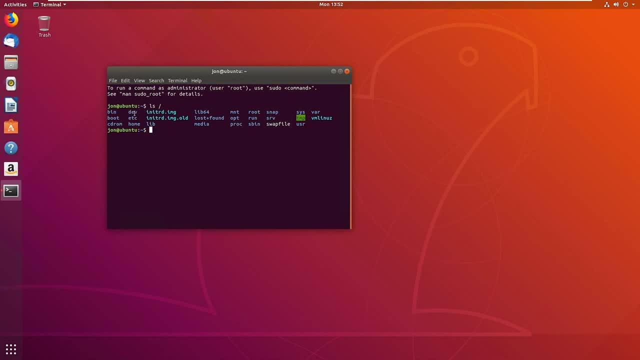 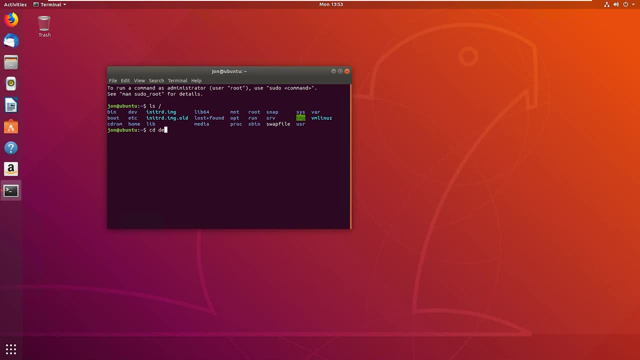 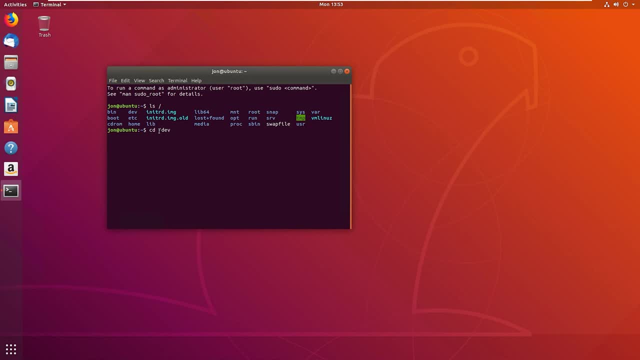 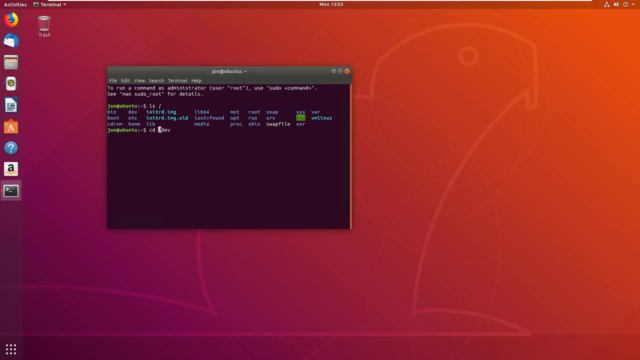 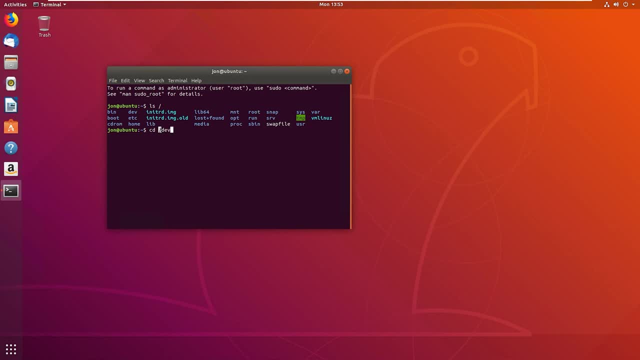 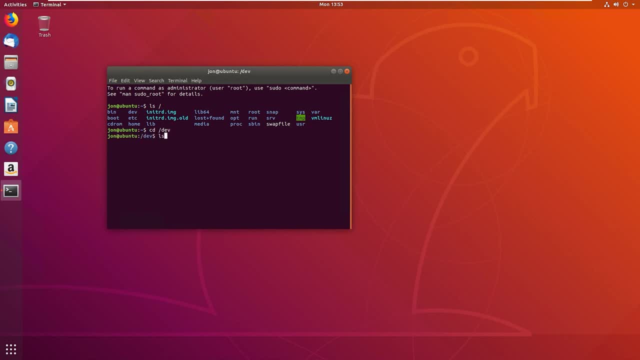 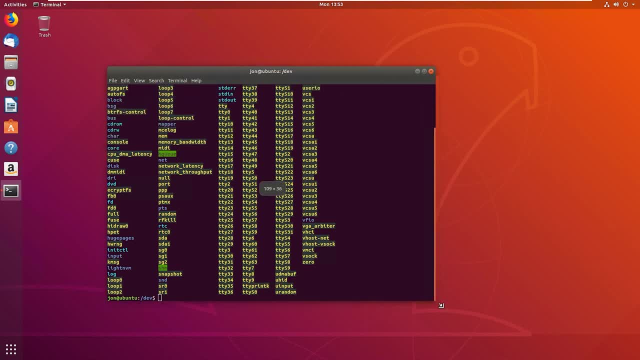 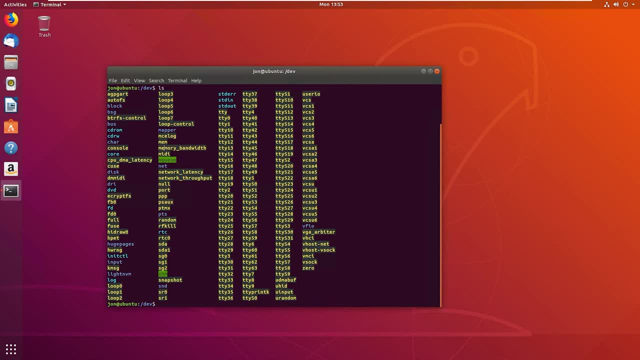 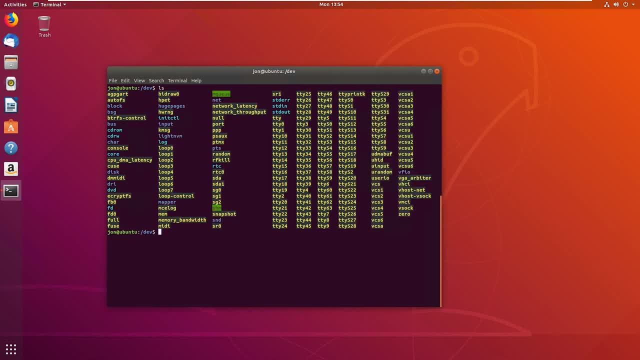 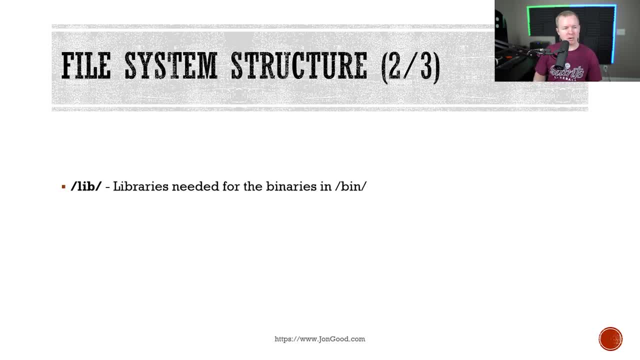 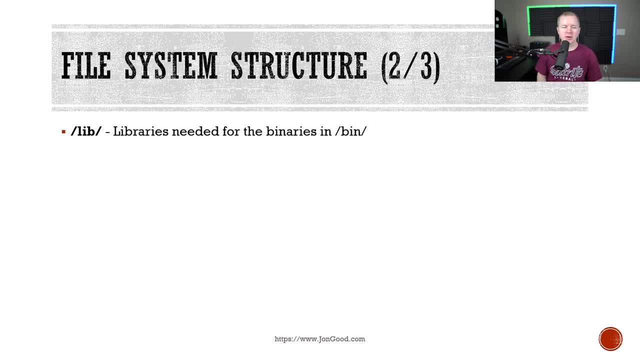 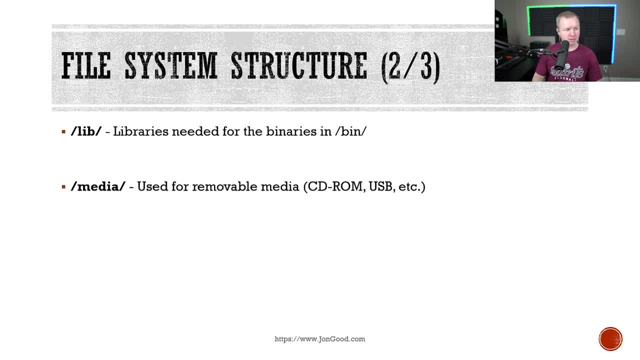 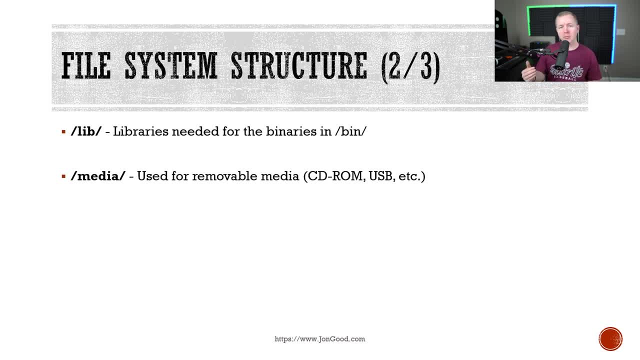 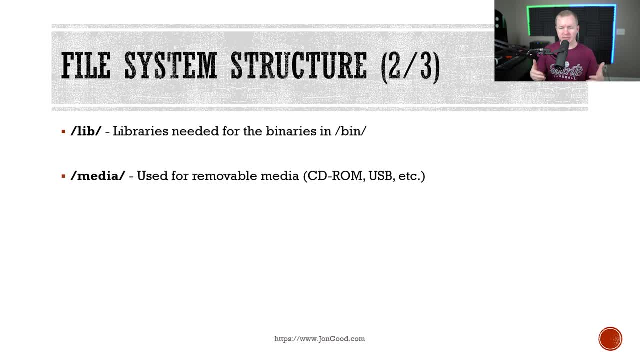 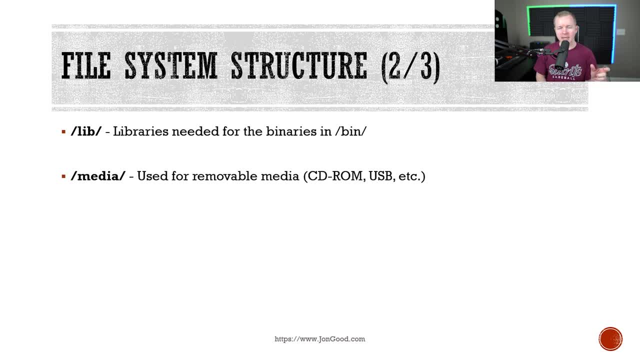 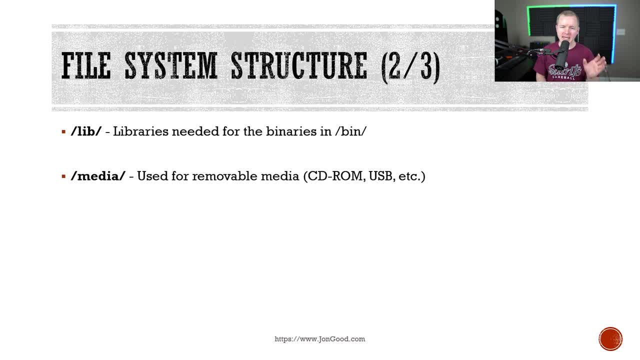 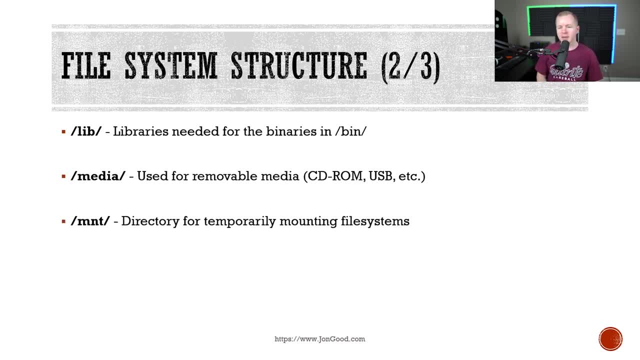 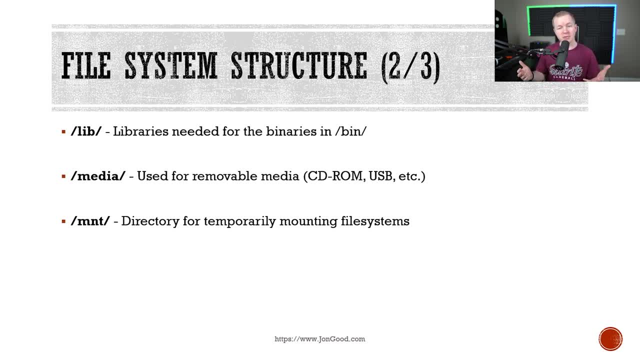 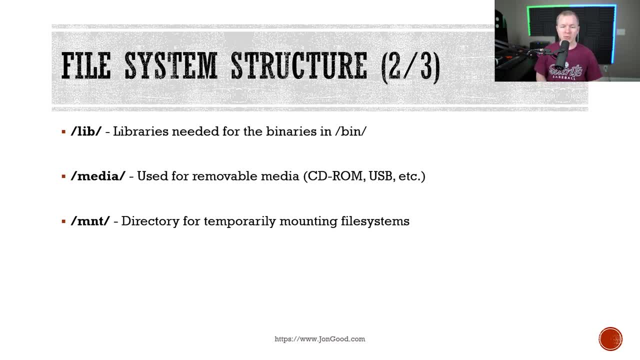 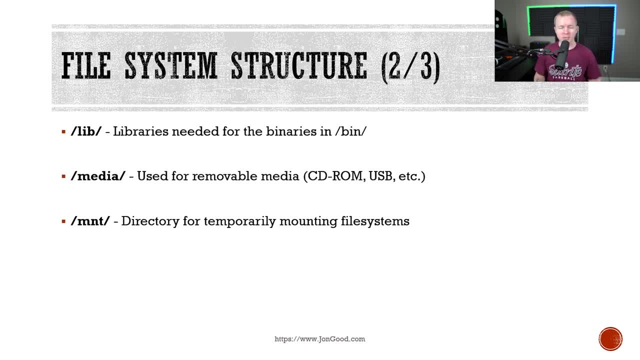 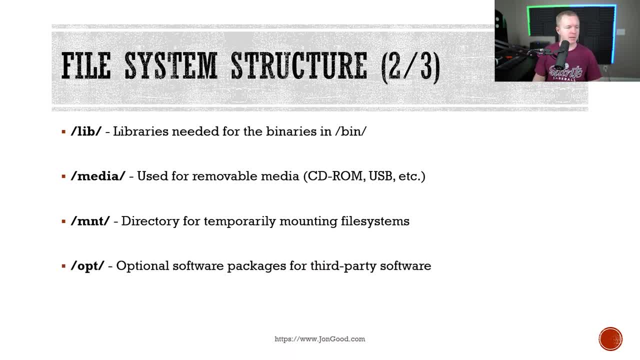 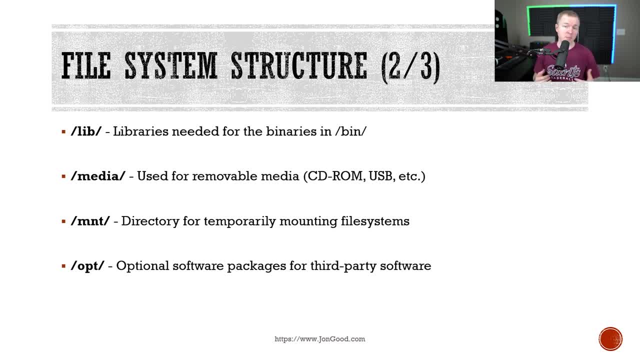 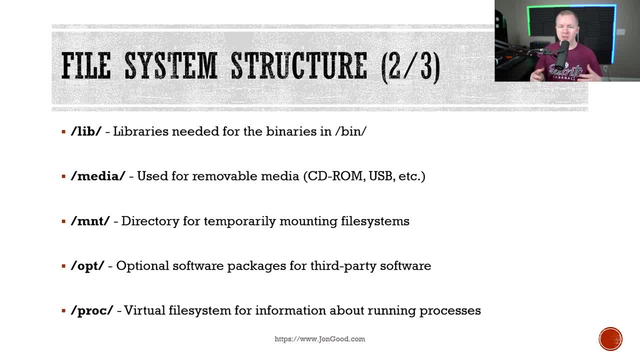 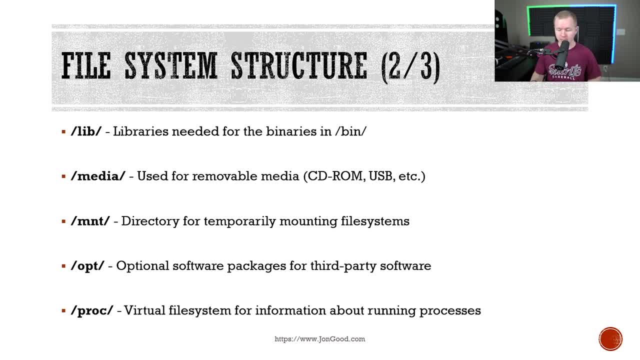 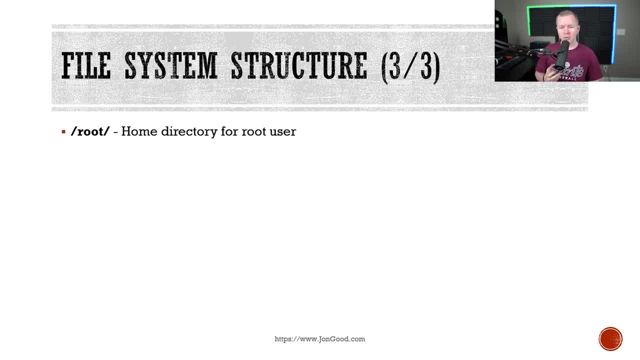 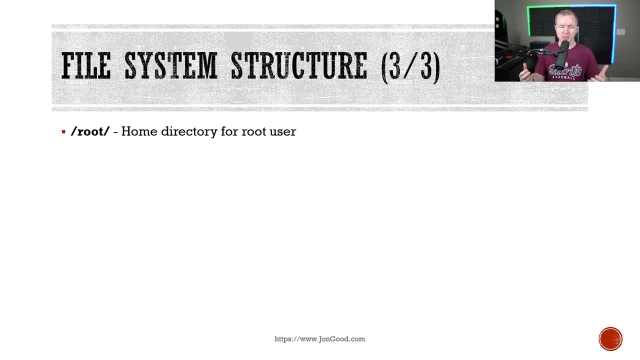 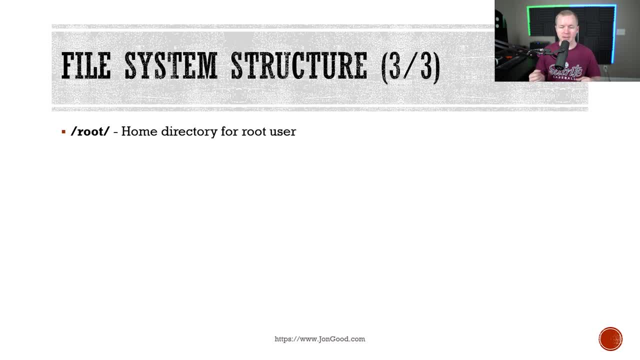 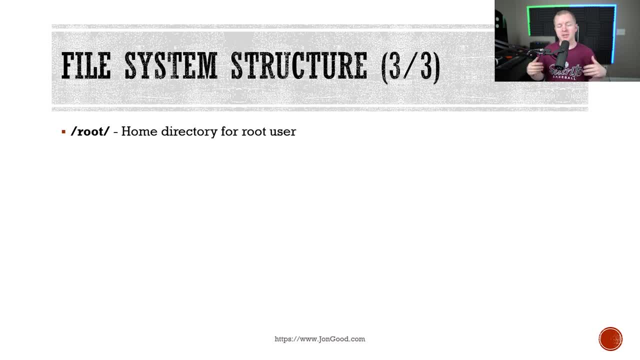 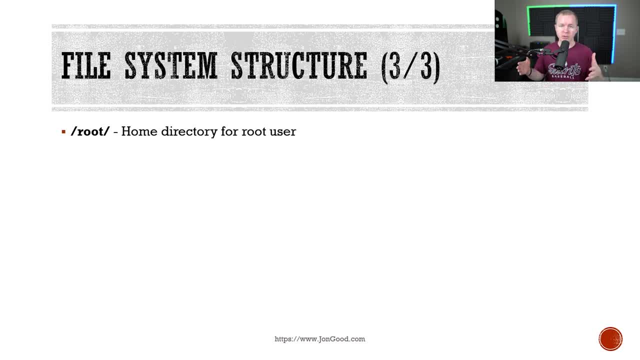 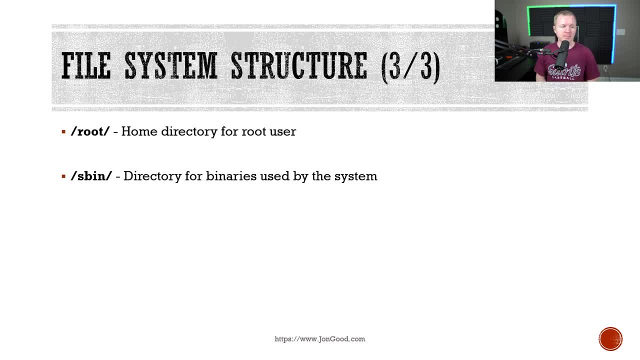 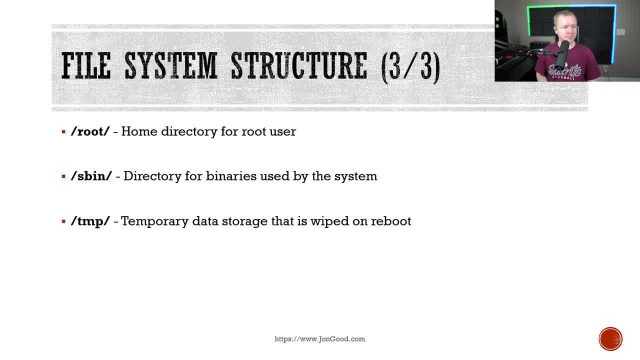 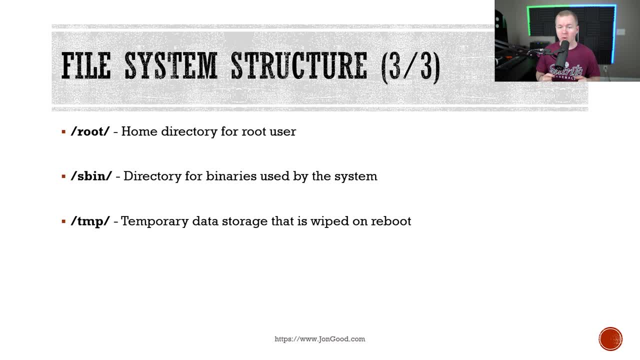 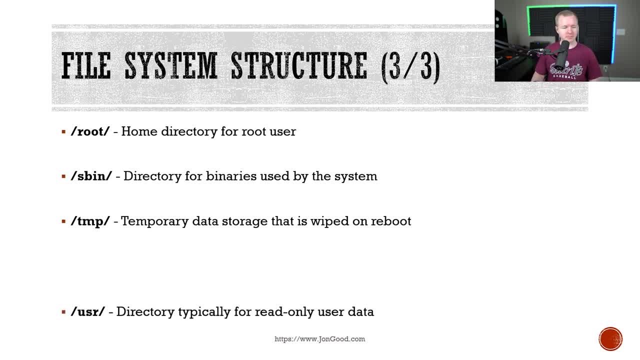 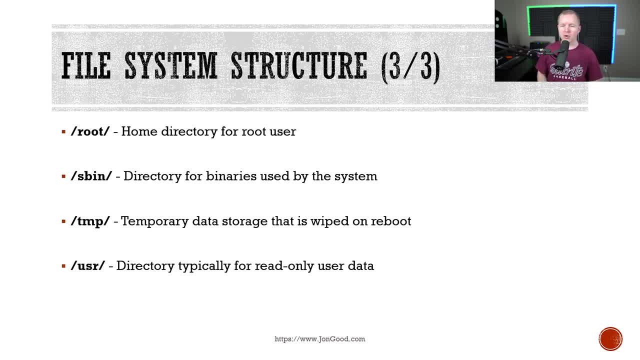 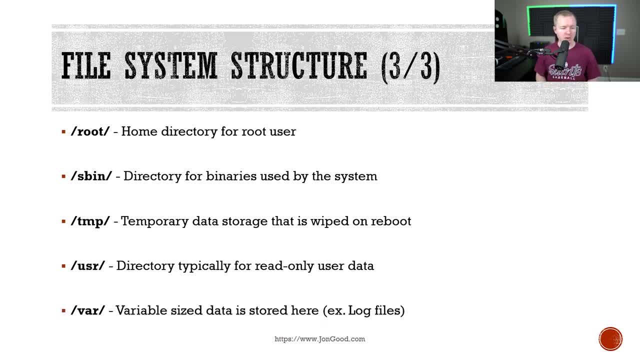 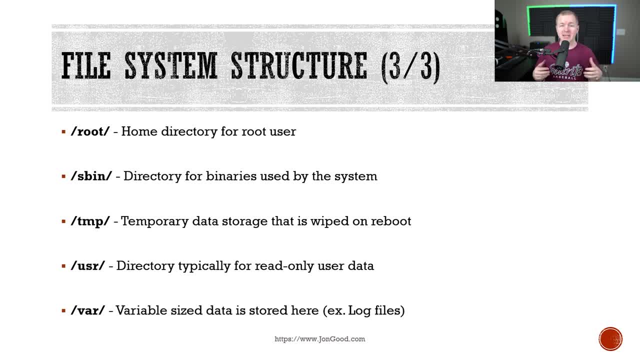 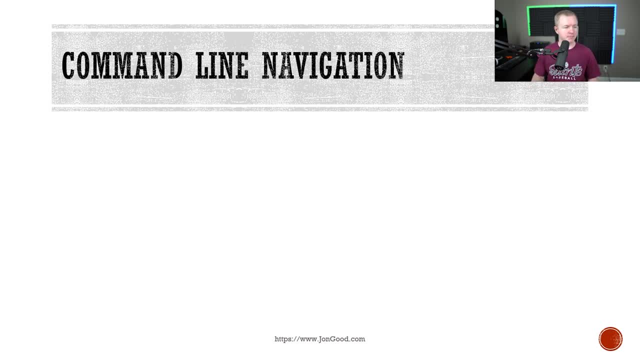 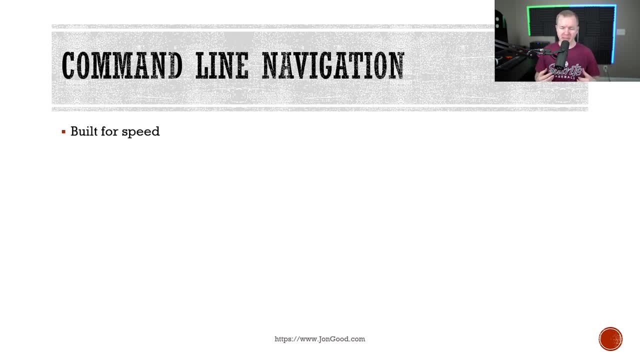 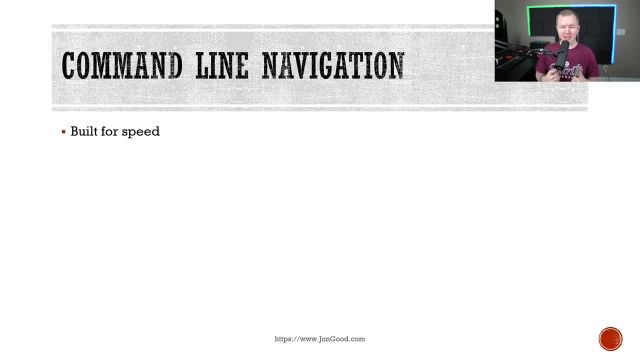 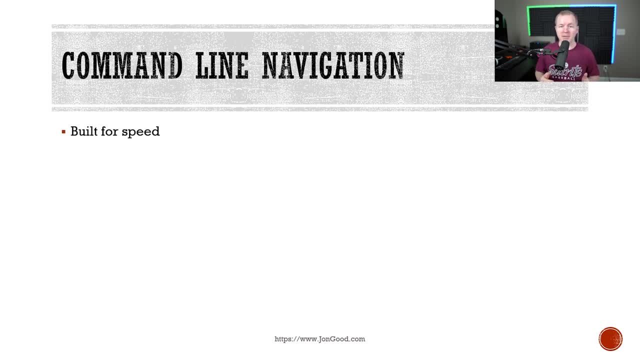 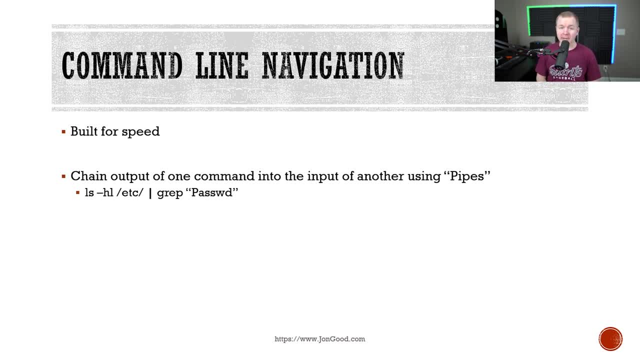 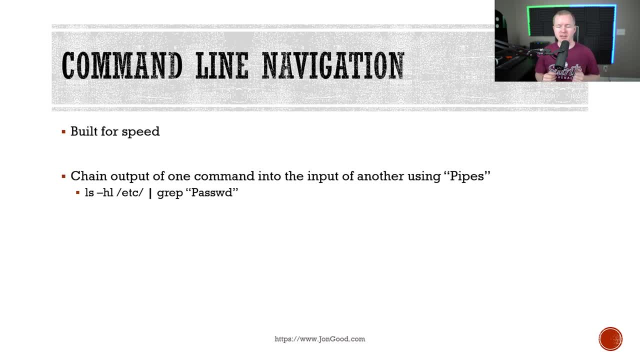 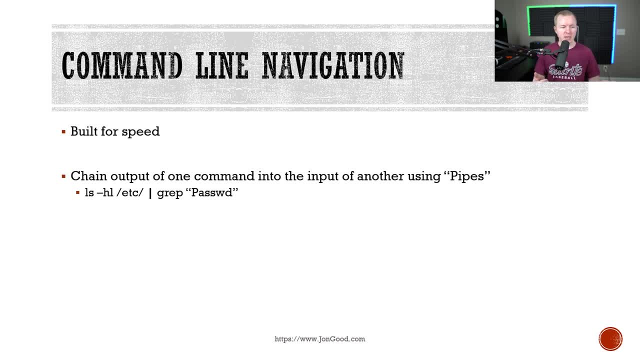 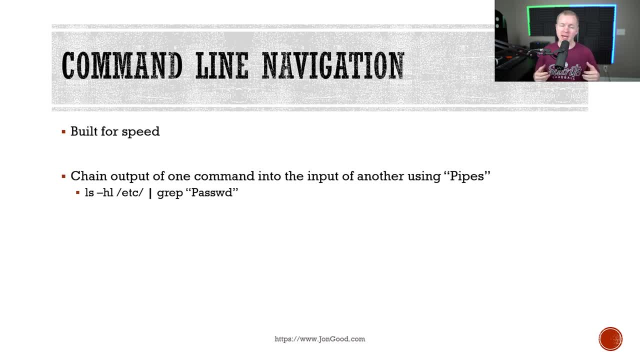 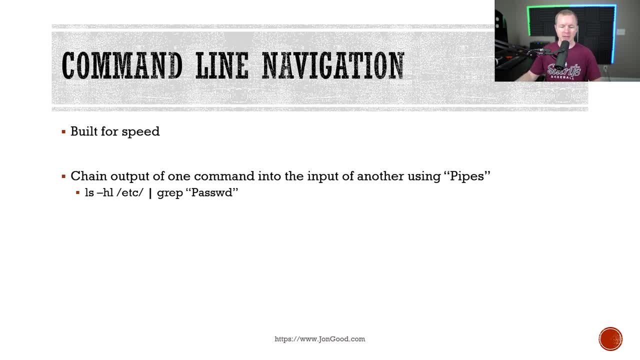 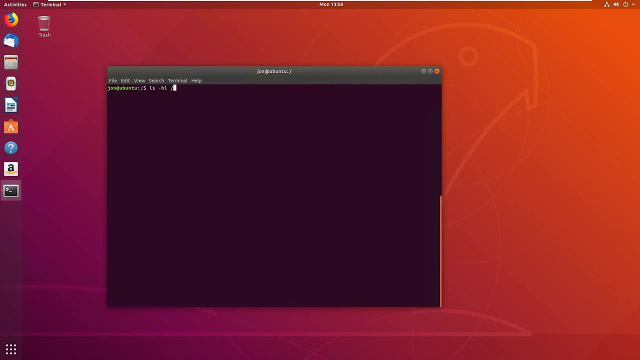 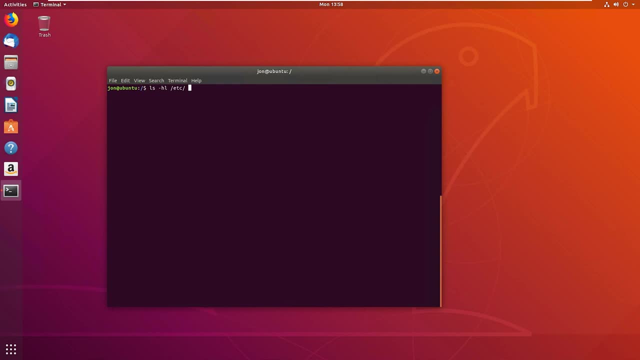 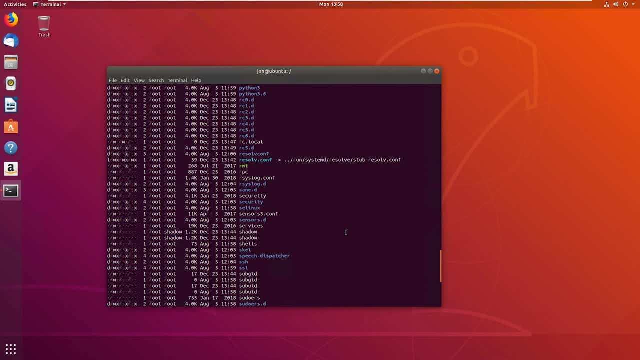 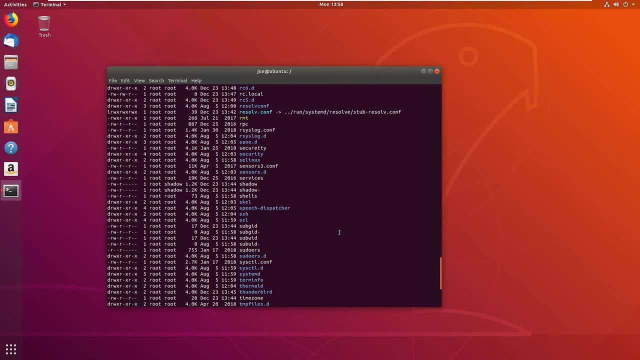 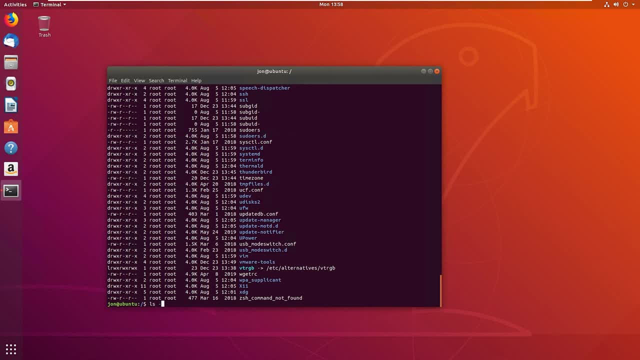 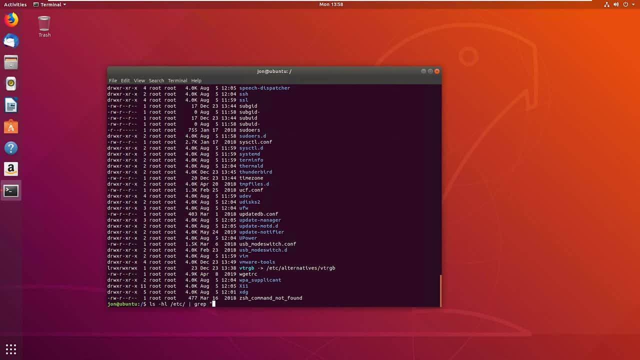 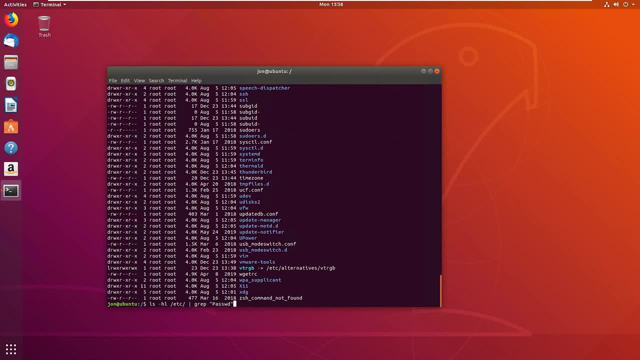 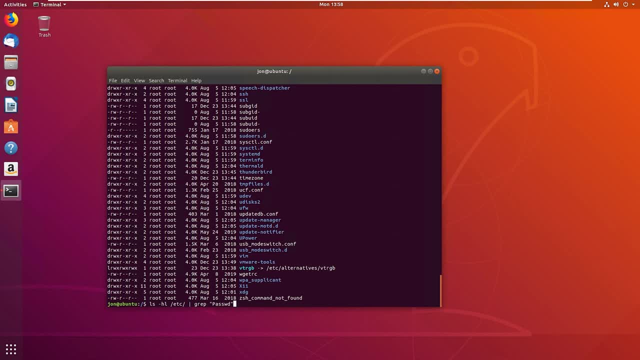 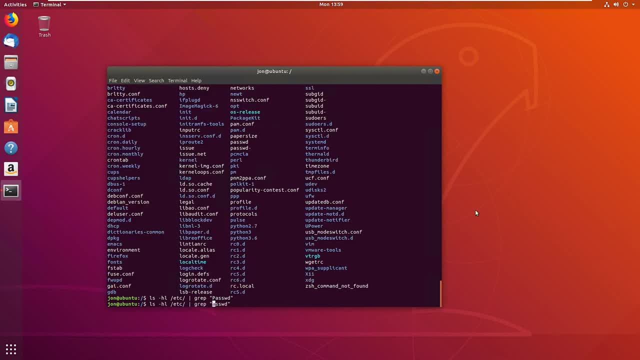 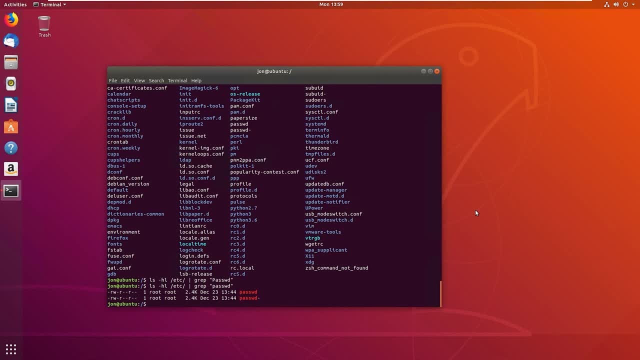 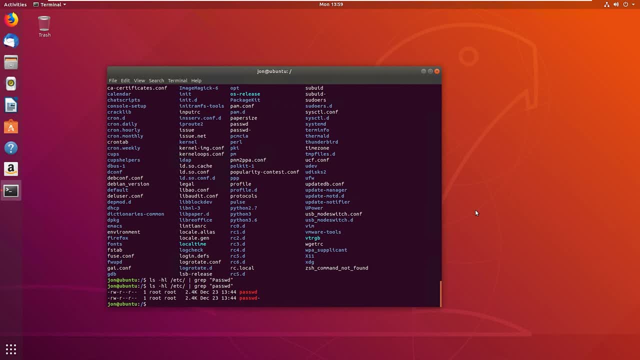 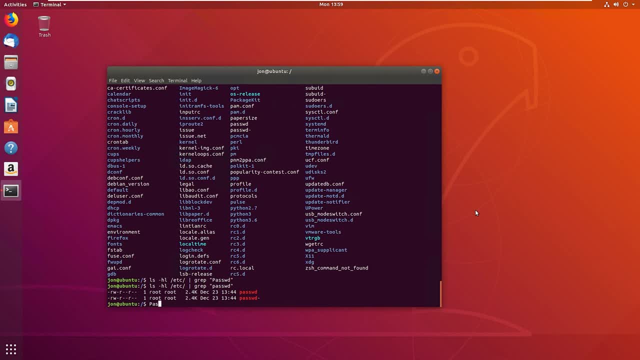 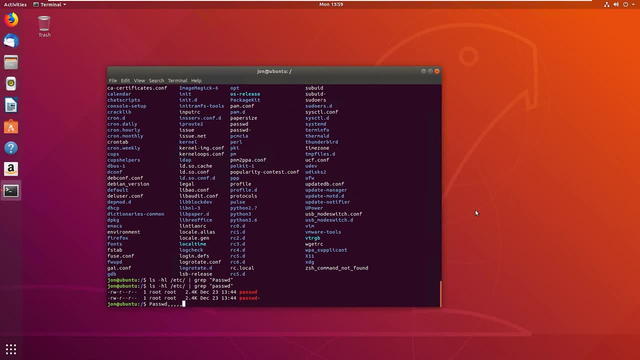 You have to type it out correctly because, as we saw, a password with a capital P is different than a password with a lowercase p, and so on and so forth. So case sensitivity is extremely important, so make sure you're aware of that. But using the command line we can chain the commands and we use the listing of the Etsy. 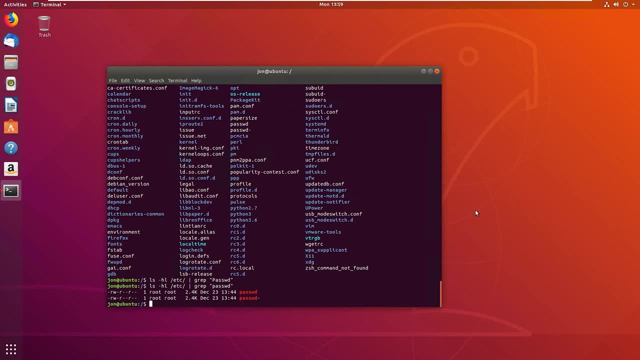 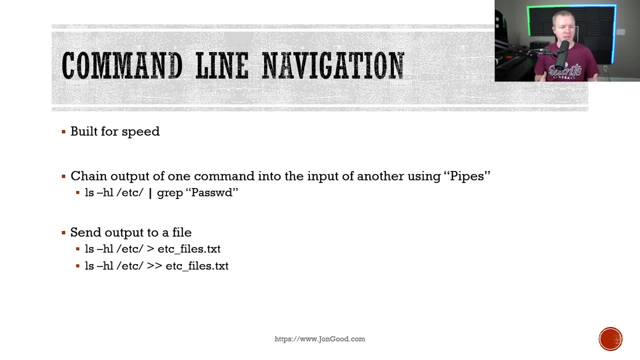 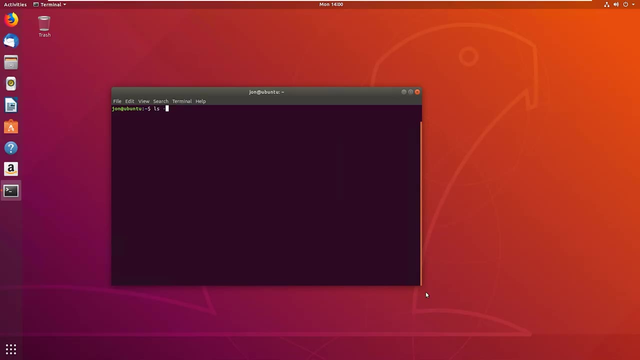 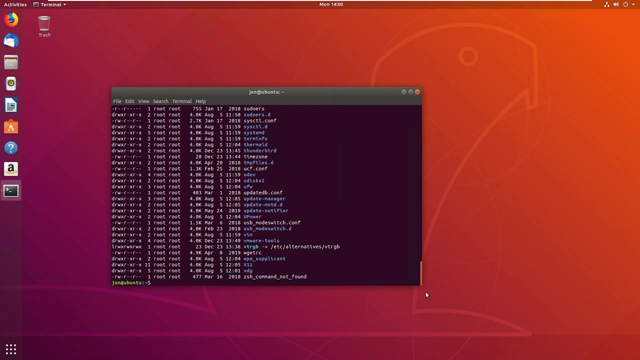 file at first command. The output of that feed into the input of the next command. okay, we can also send the output of a command to a file. let me show you that real quick. okay, now I am going to list the Etsy files that we saw here. okay, I'm going to take all of that information. 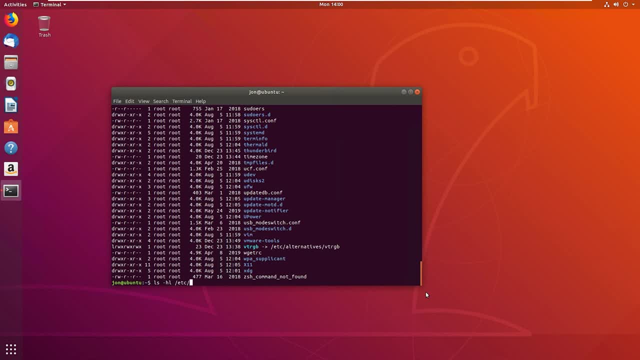 and to go back to the last command here in the command line, all you have to do is press the up arrow. I'm going to send that information into a file. okay, but we are going to call that. call it Etsy underscore files- dot text. okay, so it's. 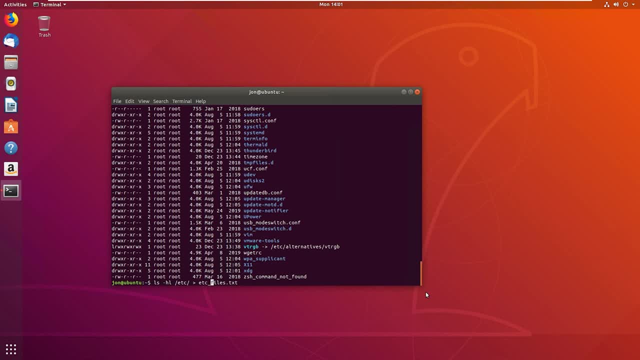 going to take that first command and it's going to create the file and send all of the information into the file. so now, when we want to read that file, we can use more, and then we're going to type that in. type that file name and you can use auto-completion. is what I just did there. 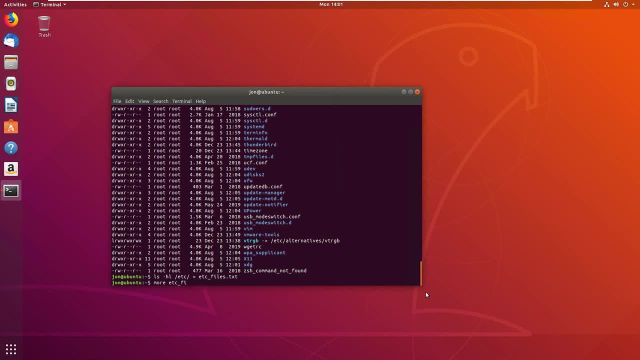 where you type partial of the word you want to type or the commander file. then you hit tab and then enter and, as you can see here, all of that information went into this file. now I want to show you this as well: the single arrow here that well, oh that we'll overwrite all the information in that file. so with 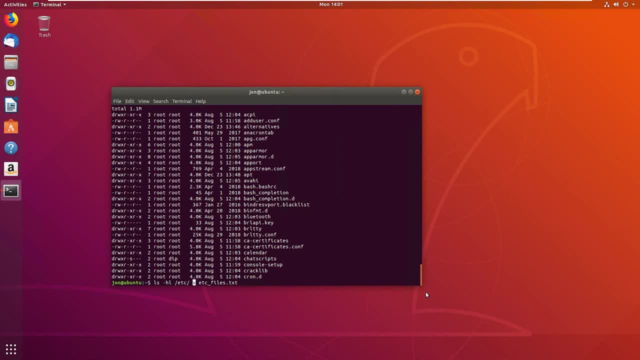 that file already exists. it's going to overwrite that information. if you wanted to append it, was you have to do is put two arrows- okay, two arrows to the right, and that will pin the file. for instance, let me show you this: so I'm in a different directory here and I'll show you that. so I'm in directory. 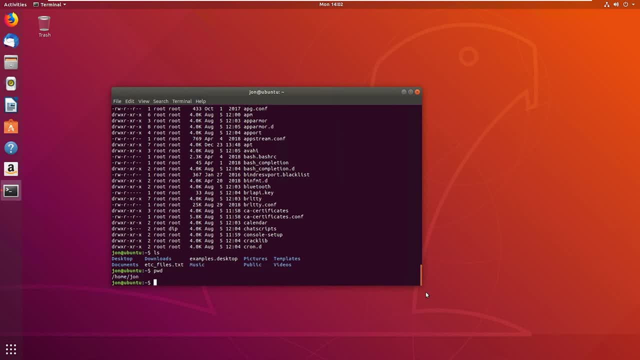 that i am in right now is the home slash job, so i am going to list the files here and i am going to actually put that into the filestxt. okay, now, before i do that, let's remember here: this is what's in filestxt right now: all those etsy files. so i'm going to list out everything in this current 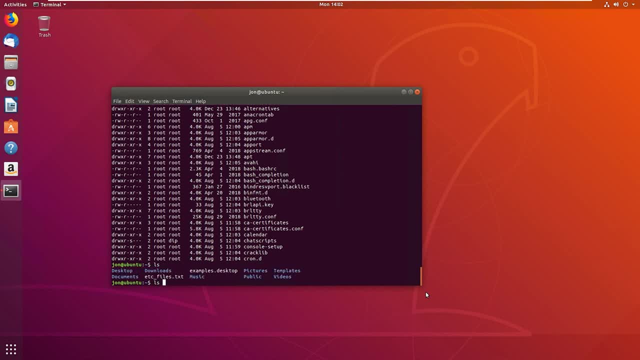 directory which is this information here, and i am going to send that to the etsy filestxt file. okay, now we're going to read that file. as you can see, it's different. that single arrow, it overwrites everything that's in there. now, if i wanted to append all that information, go back to that same command, but we're going to. 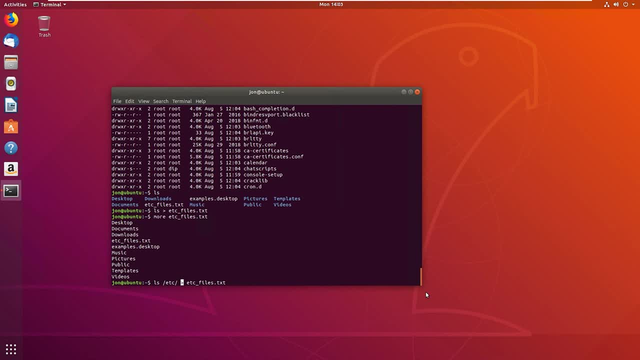 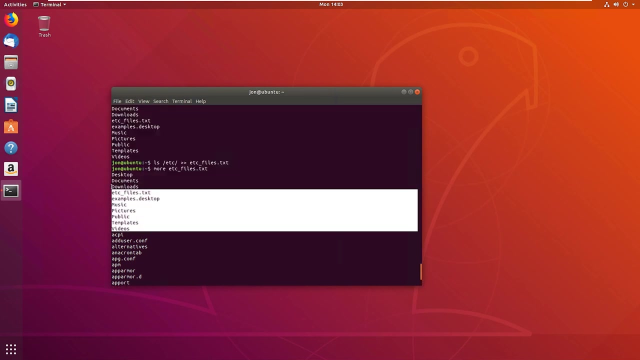 list all the files in the etsy directory and we are going to append to that file. okay, so we do that, and then we go back and we read that file again. now you have all those other files in there. okay, the beginning here up there, all this whoops, all of this stuff is from that directory that we're 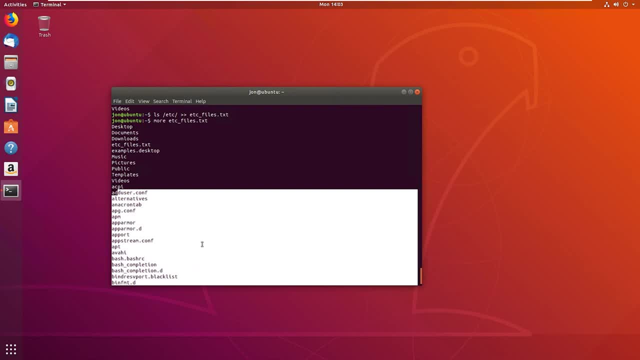 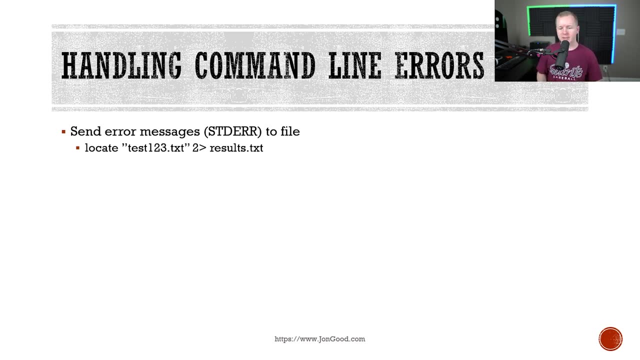 in now and then it appended at the bottom all this other stuff. now there are ways to handle command line errors that you might receive. maybe you want to send them to a certain file. you can send the error messages to a file using this command. here, for instance, if we were using 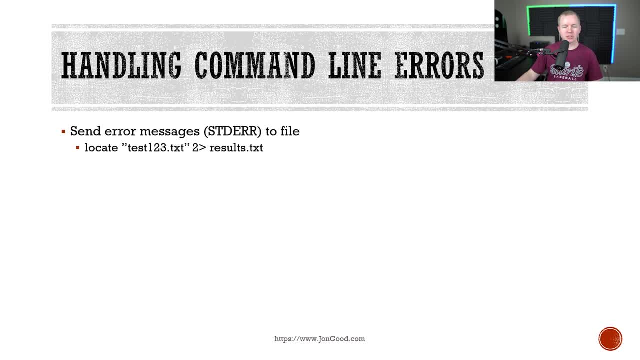 the locate command. we can use the two and the arrow here to send that to a file. if we want to send the errors and the output to a file, it would use the arrow and the ampersand. now, navigation and file management. pwd is an important command. 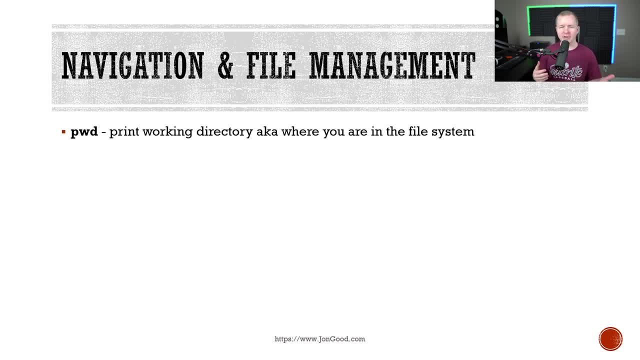 because that is going to show you exactly where you are in the file system. it's going to show you the folder that you're in right now. cd changes directory to another location on the file system. ls lists the files and folders in the the location that you're at or that you've specified, and then ln creates a shortcut or. 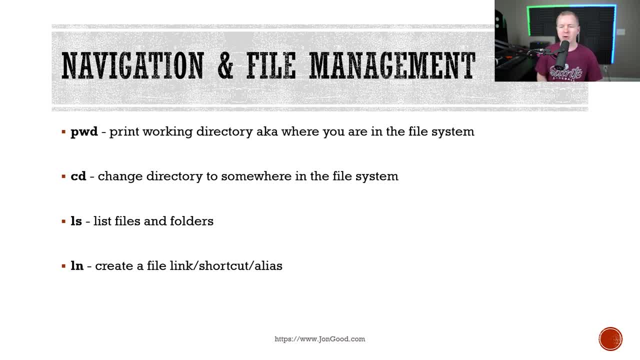 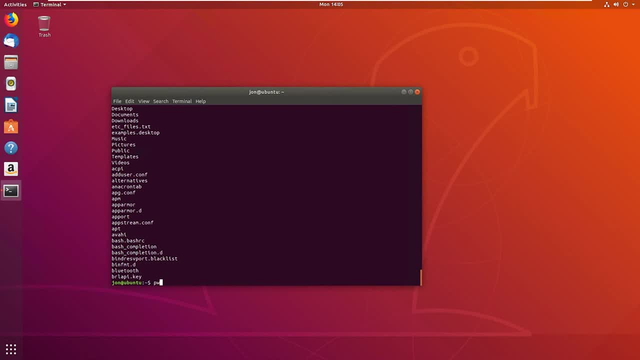 alias, just like you would on your windows computer or any other computer. i'm going to show you a few of these on the command line here. so again, we've already used several of these, but pwd shows us exactly where we are in the structure. so if we were to change directories to the root and then 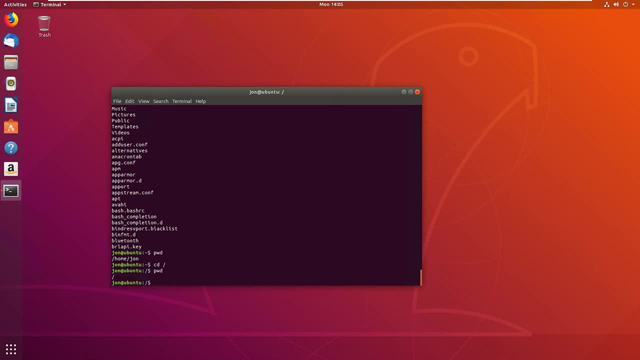 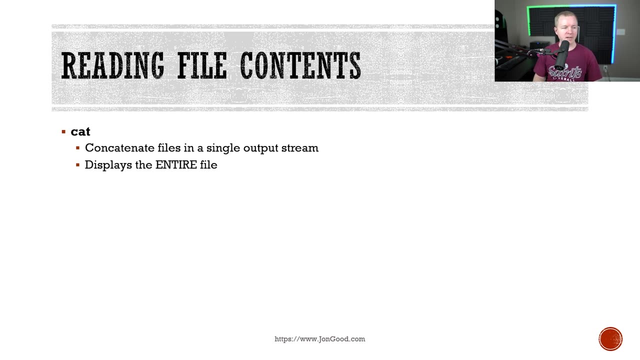 we did pwd, it will show us the slash, because that's where we're at now. and then, of course, we've used ls already and you can list the files reading file contents. so we need to be able to read files throughout the linux operating system. so one of the first commands that you learn when 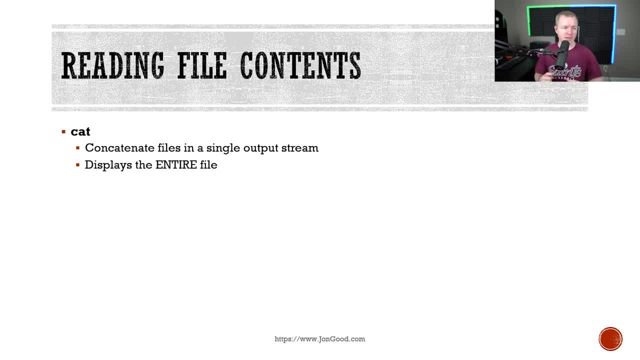 you're talking about reading files is the cat command. cat will display all of the information in a single file. think about this. you've already kind of seen in the demos: if you have a very long file and we use the cat command, that will spit it all. 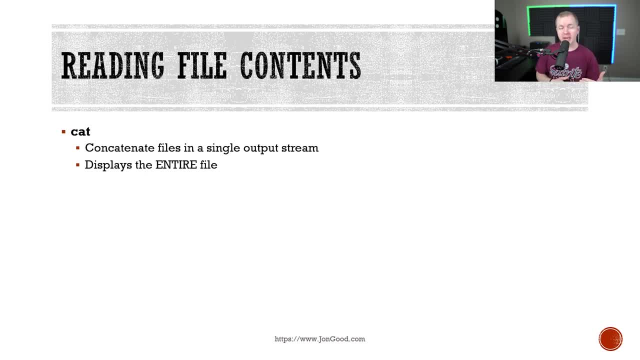 out at once. it makes it very hard to consume information on a large file. it's actually an older command as well, or more is a way to read the file contents one page at a time, and then you also have less, and there's a joke that less is more, but basically, 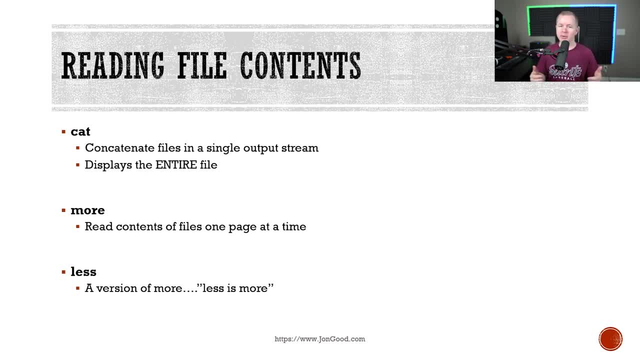 it's another version of more, so it will do it page by page. i highly recommend you use more or less commands, generally the cat command. it's not going to be useful, especially if you're reading large files, because you're just you're going to have to scroll through everything. it's not going to be. 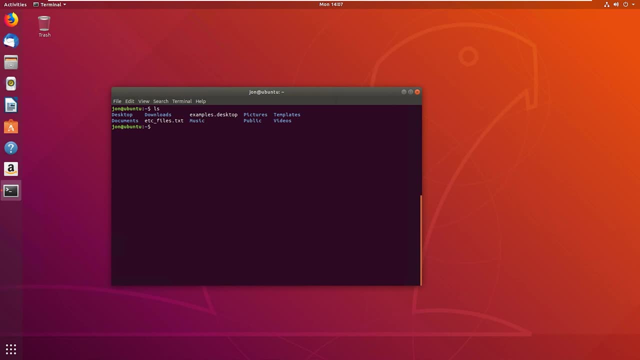 useful, so i'm going to show you what the difference between them are. so if we do cat on the etsy file file that we already have, see, this is everything in there. it goes to the very bottom, so all of this information is in there, okay, so that's a lot. 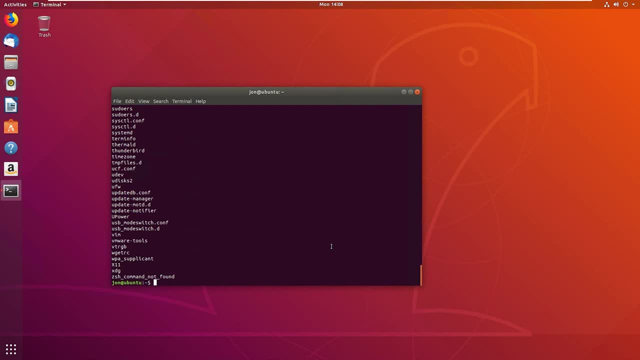 that's that makes it hard. if it's a really big file, we can use the more command oops and we can use the space bar to go page by page and you can see that there's a progress bar on here too. through the file makes it a whole bunch easier to read that. and then we can also use the. 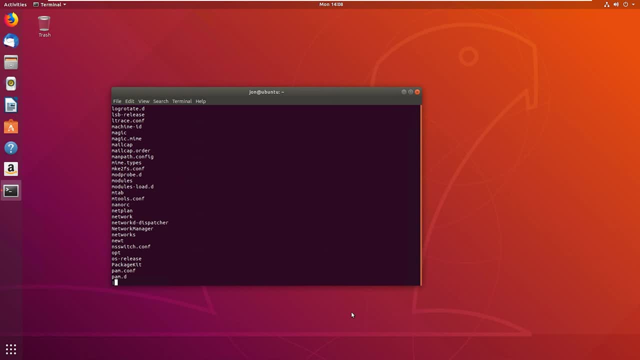 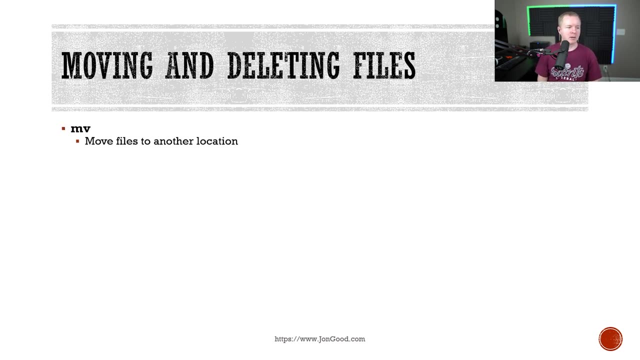 command as well, and the same thing. you can hit the space bar and it goes page by page. now let's talk about moving or deleting files. so some of the commands around moving and deleting files. you have the move command, mv, and then you can move files from one location to another. 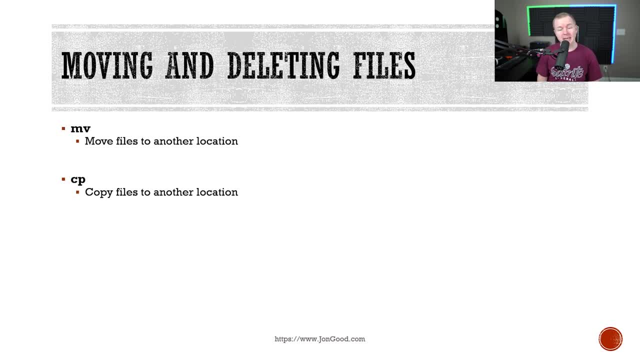 we have a copy command, cp, and this copies files from one location to another. we have the remove command, or rm, and that removes a file, just like deleting a file. and then we have the rm dir. rm dir- we're removing a directory. now, what you'll want to do if you're 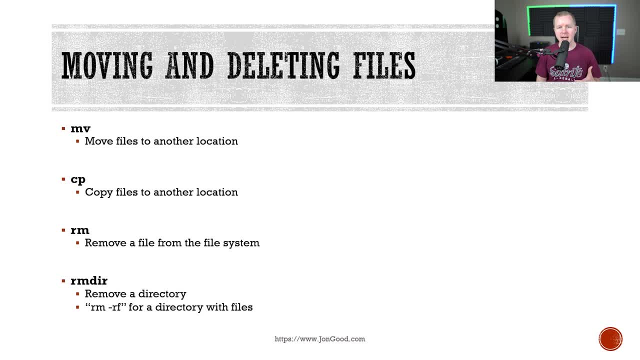 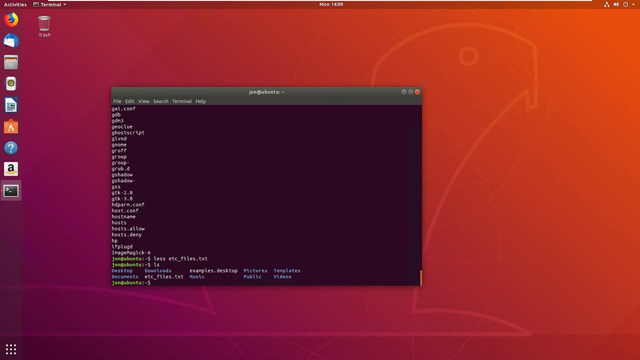 using the remove command. you would use rm, dash, rf and then the file, the folder, to delete everything with inside, because it recursively will delete everything. let's go to the demo here. we can move this etsy file to the. move it to the desktop folder. so we're going to move the etsy file. okay, to the. now here's an. 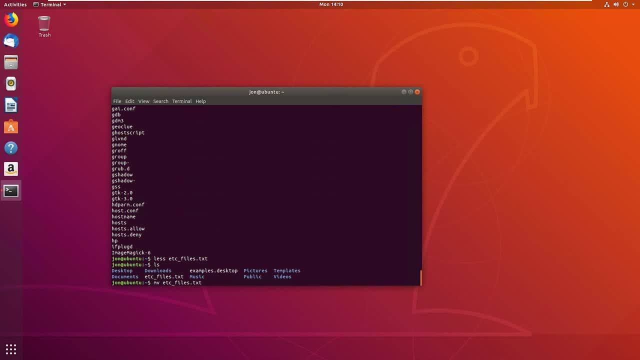 interesting thing too. since i'm already in this folder in this location, to move it to the desktop, i would move it the desktop, like that. okay, we don't put a slash in the front here, because remember that slash represents the root file system, the root of the file system. so if we put a slash in here, 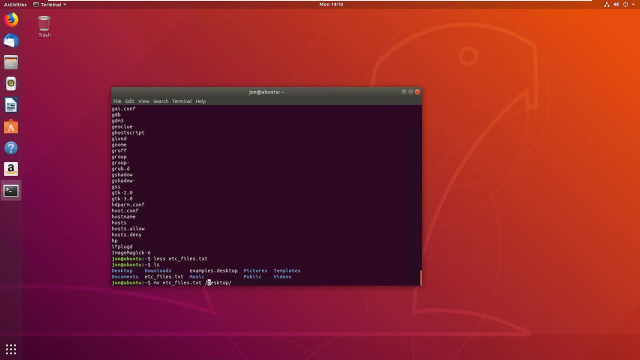 there would have to be a folder called desktop in the root of the file system. if you remember, we are actually in the slash home- slash john folder, okay, so that's an important thing when you're dealing with files. so we're going to move the etsy files into the desktop folder. 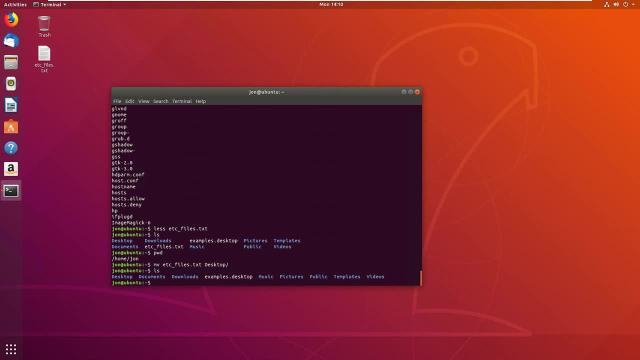 okay, now you'll see it's no longer here. we're going to change directories into the desktop folder and we're going to list the files and then there it is. okay, now we're going to copy the file. so copy etsy files. we're going to call it etsy underscore files. underscore two dot txt. 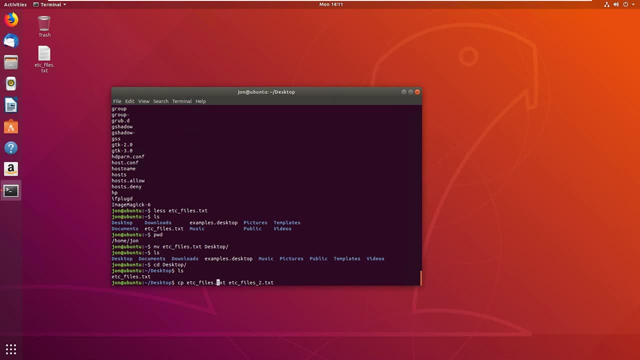 so the original file and then what we're going to name it. okay, now we're going to list the files again and we have an exact copy of that etsy files folder. now something interesting, because i have several files that are named the same thing. if i type, start typing one file name or one folder name. 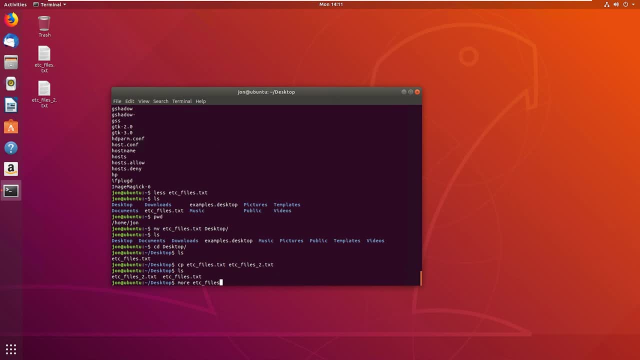 and then i try to tab complete. it will get the majority of what the files are named and then it will stop there. so then you have to further describe what you want to use. so i'm going to hit buy copy now and you're going to create a file scroll. 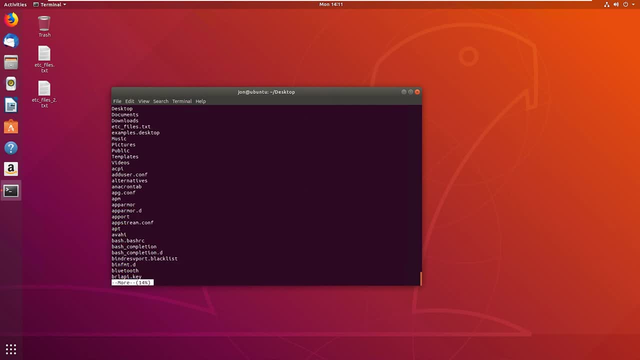 going to do underscore two and then press tab and then it will go through. okay, so an exact copy. now we're going to remove the etsy files to file. so rm etsy files. remember, i didn't fill it all the way in, so i need to do underscore two. 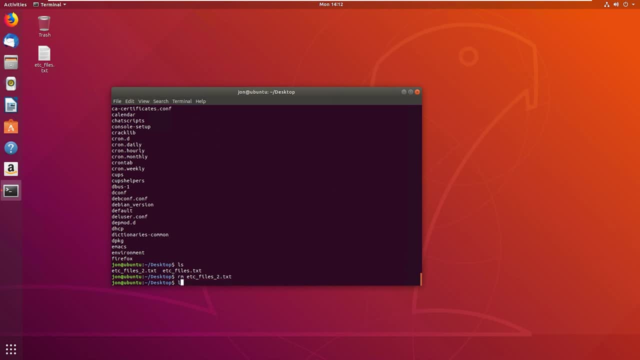 and that is going to delete it. it is no longer on the file system. now we're actually going to create a directory, which was not on this list of commands, but the command to make a directory is the mkdir. so we're going to make a directory and we're going 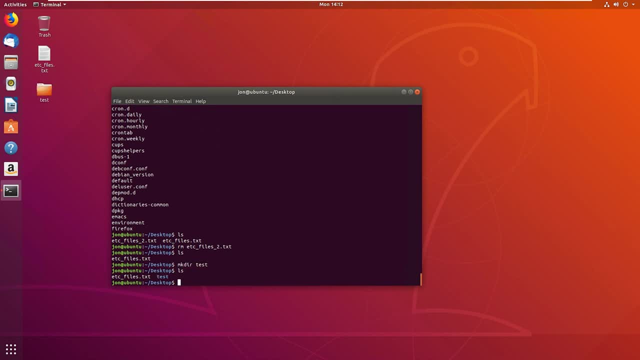 to call it test. okay, so now we have a test directory. now we are going to move the etsy file into the test directory. so type test tab. so now in the test, whoops. and then again that's what i was talking about, where you can't type a slash in front of a file or a folder. that's in the directory that you're in. 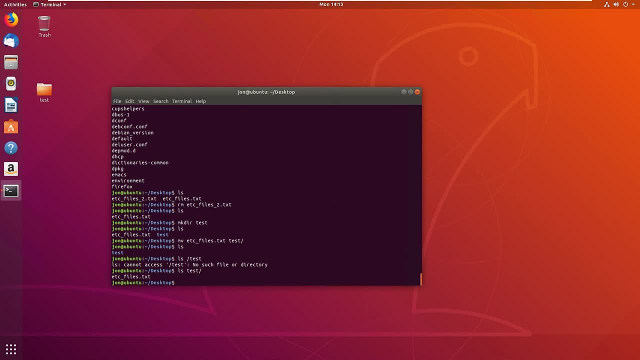 right now. so we're going to this out the test folder and there's the etsy files. now we're going to remove the test folder. so rm dash, rf test. now i'm going to show you this real quick here before i do that, what it says. so if i try to just 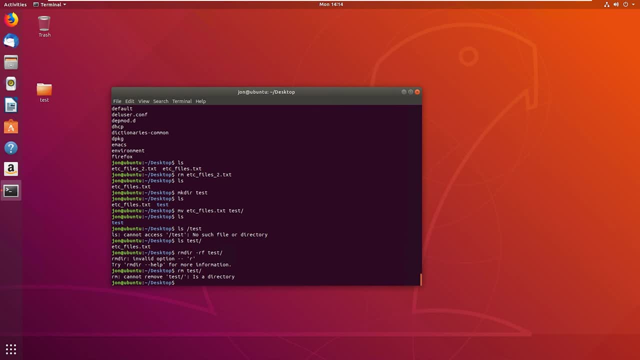 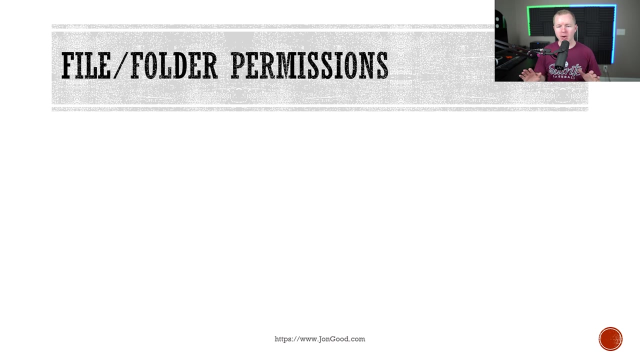 do rm, it's actually going to say this is a directory. i can't do it. and then if we look inside there, the file is still in there. so i'm going to do rm, dash rf test and that just deleted the folder. now i want to go over the file and folder permissions that you need to know. 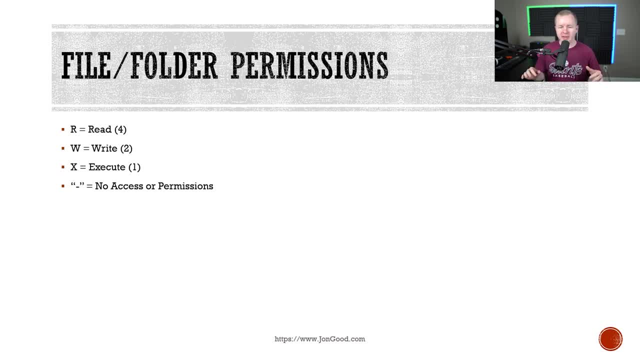 so with linux it's going to be a little bit more complicated. so i'm going to go over the file and folder permissions that you need to know. so with linux it's going to be a little bit more. the file permissions can be kind of confusing because they aren't exactly user-friendly as far. 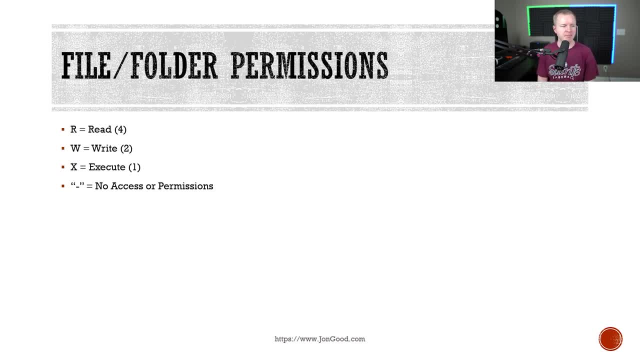 as initially learning them kind of different as far as the scheme. so you have three different types of permissions. you have a read, you have a write and you have an execute. okay, those are three types of permissions, so they can be an r, a w or an x. now 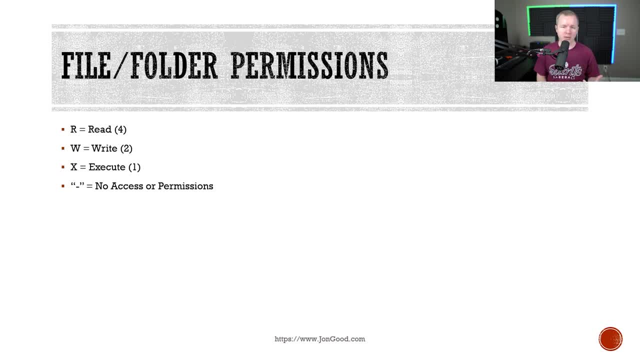 you can see that the file permissions are kind of confusing because they aren't exactly user. they also have a numeric representation. so read is four, right is two and execute is one. permissions are added up when you provide multiple permissions. so for instance, if i give somebody read and write, it is going to be four plus two. you can have a maximum of a number of seven. 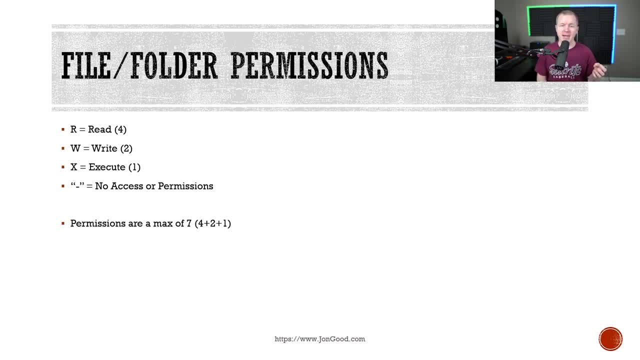 for the permissions and that would be read, write and execute. an example: if we have permissions of 754, okay, the first number is the owner. so the owner in this file has a seven. that means they have read, write and execute r, w, x, four, two, one. okay with me so far. 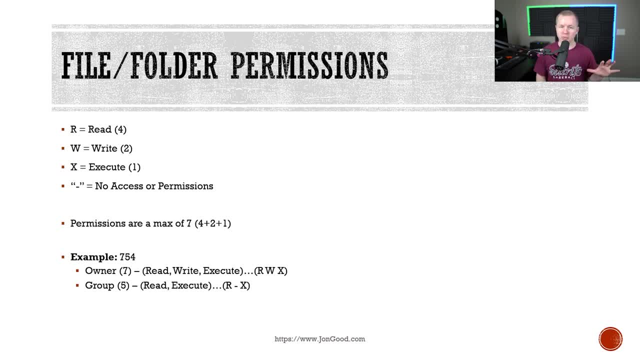 the second number is for the group, so every file and folder gets assigned a group. the group in this case has a five, so a read and execute r and x. four and one. the last number is for the world, or everybody else. okay, it has a four, that means read. 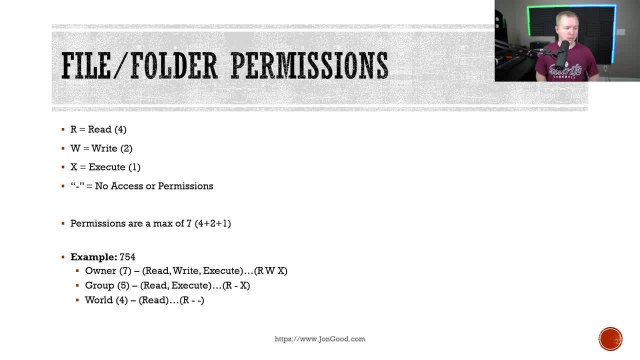 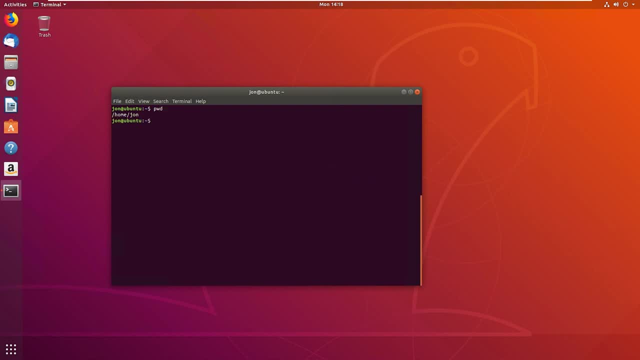 or r or four. right, i'm going to create a file here. i am back in the slash home, slash john directory and we're going to use the ls function here. we're going to call it testtxt. okay, there we go. so if i want to see the permissions on that file, i can do ls. 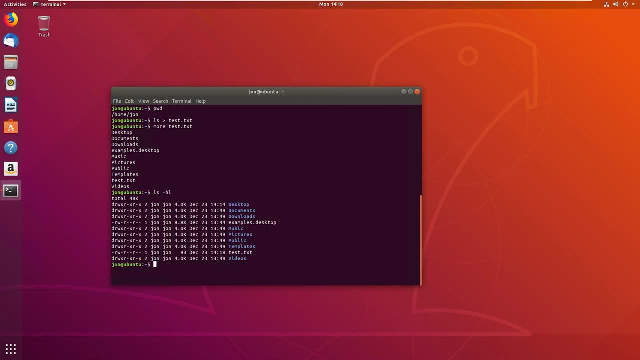 hl is usually the one that i will do. that will show all the permissions. okay, this is the testtxt file right here. okay, so each level, the owner, the group and the world or the everybody else, three dashes here. okay. so for the owner, we have read, write and there's no execute set on this because it's not a script. 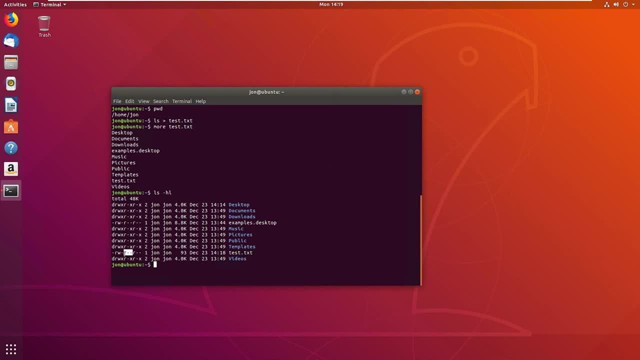 or anything. well, we have set the Benson document here in here. which is the owner? okay, so we see how this and the rule set is unclear. gotгу group has read nothing. another in the world has read nothing. rather, or then, how you look at it here is: this is the user, this is the owner. 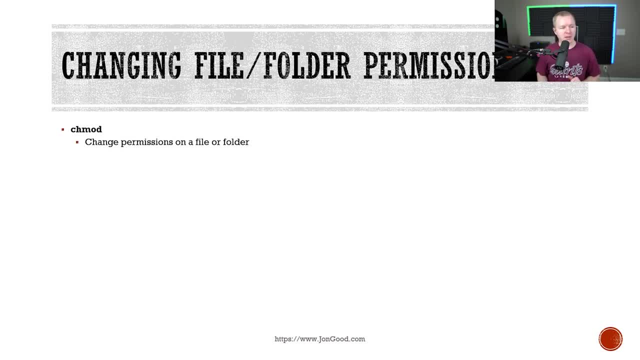 and then this is the group. now what happens? if we want to change the file folder permissions, how do we do that? let's go into that. so you have a command called Tchamad. that's what you use if you want to change the permissions on a file, world log pen or something like that and other in there. so you walk back to the screen here, which is秦, and you move this and a group over here. 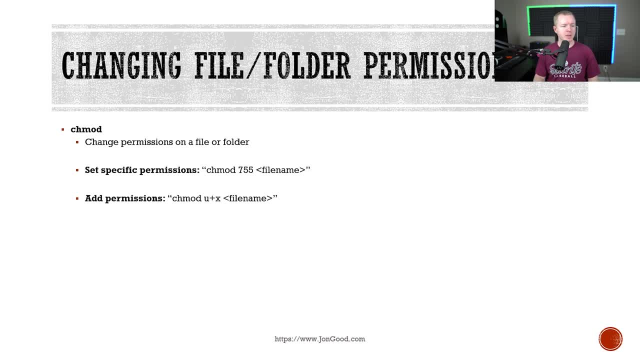 on a file or folder. If you want to set specific permissions, you can do chmod, for instance 755 on the file, and that would give the owner read, write and execute Group would have read and execute. Everybody else would have read and execute- 755.. 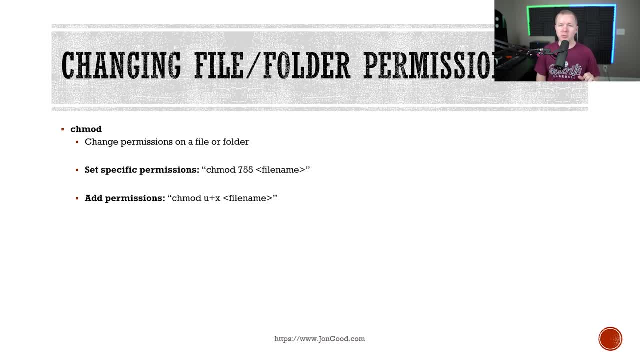 You can add specific permissions as well. So if you want to change a file into an executable file, you can do chmod, and in this case it is the user, so you plus x for execute and then the file name. 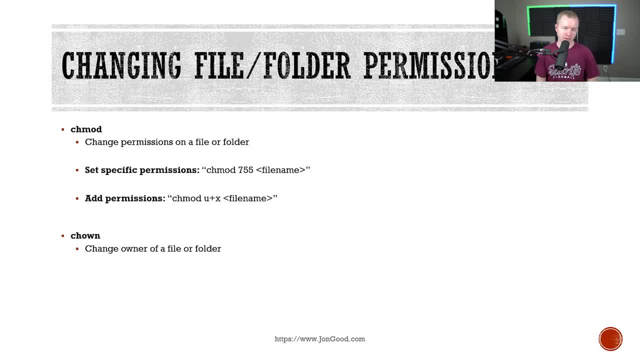 Chone changes the owner of a file or folder. You want to change the owner? you would do chone the username and then the file name, Okay, and then you can change the group only. So chone, colon the group name and then the file name. 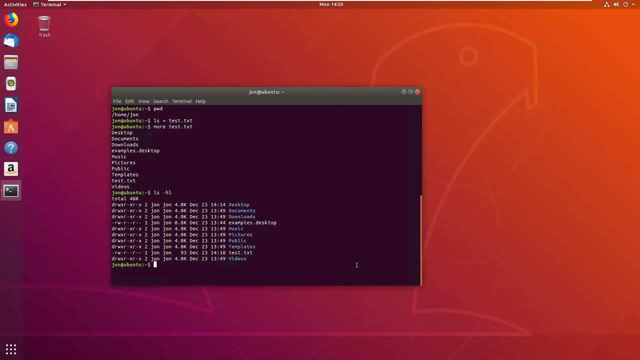 So let's go over to the demo machine here and let's do this. We're going to change the permissions on the testtxt file, So let's change it to all permissions for the owner. for us, We'll change it to a five. 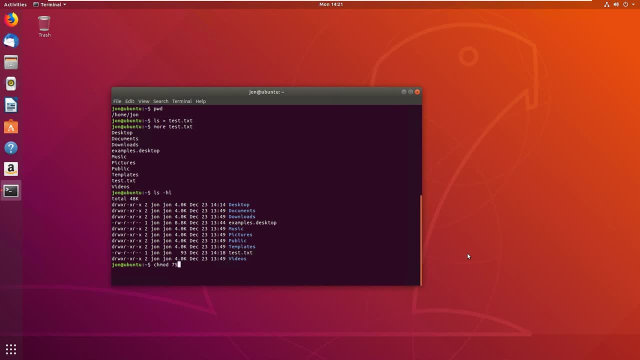 which is read and execute for the group, and then we'll change it to a zero for everybody else. and then the file name. Now let's look and see what it is. Okay, so, as you can see, it turned green here because it changed it to an executable for us. 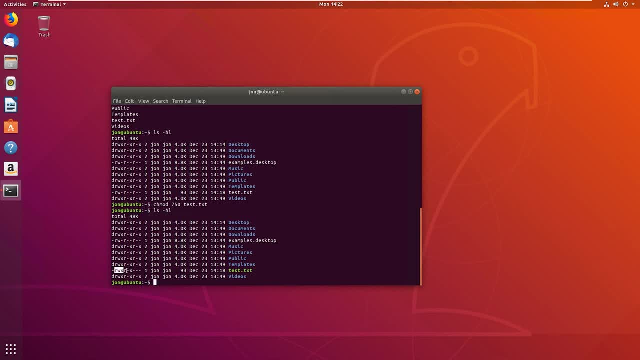 but now you have read, write and execute, The group has read and execute, Everybody else has nothing, As you can see here, this was the original. So we originally had read, write, Group had read and everybody else had read. 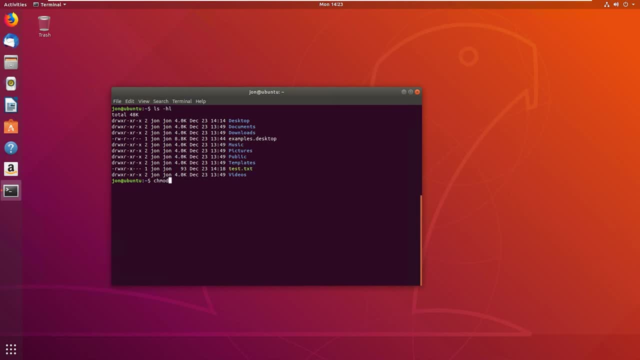 So now we're going to change the file back, So we'll do chmod. We had it at six and then four, four, Okay, so now we'll see the permissions are back to read and write for us, read for the group and read for the world. 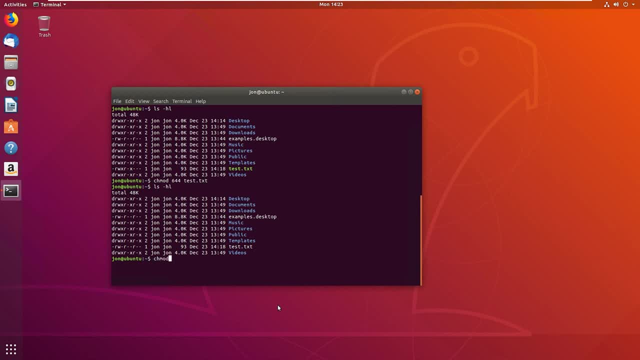 Now we're going to turn this into an executable by adding individual permissions, So chmod u plus x and then testtxt. Okay, now you can see we have changed the testtxt into an executable file just by adding that individual permission. Now we're going to change the owner of the actual file. 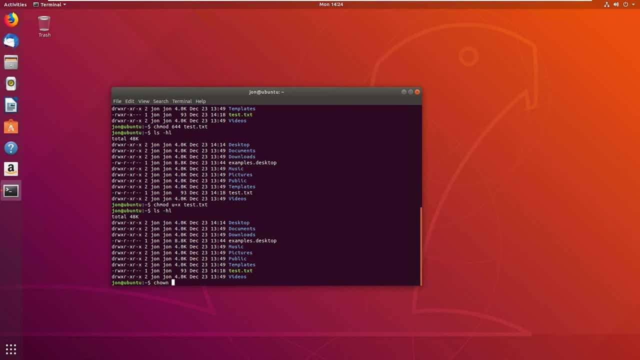 So we're going to do chown, We're going to change it to root and then testtxt, And we might have to do sudo here Now. I use the sudo command because there are commands that you're not going to be able to use. 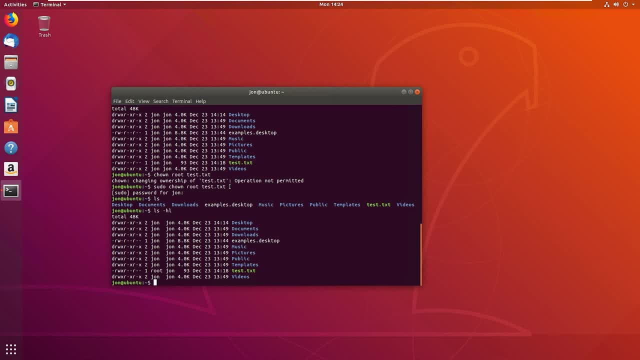 unless you're in a certain privilege level. But basically, sudo allows you to run permissions and privileges as the root user, So I had to do that in order to change that file to a root owner. That's just because of how the permissions are set up right now. 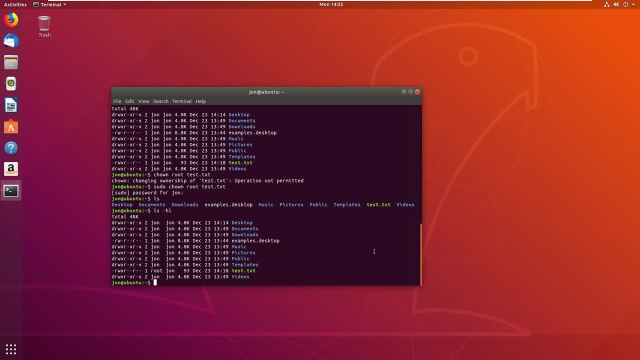 Normally, in a real environment, you probably won't have that ability, but it depends, especially if you're in like a development environment. Now let's change the, Let's change the group owner. So we're going to do chown. 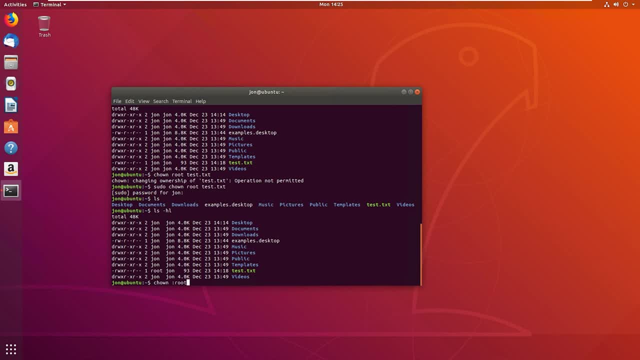 We're going to change the group to root. I think there's a root group on here, So remember colon root and then testtxt. Again, we have to do the sudo command here, So let's do that Now. this used to be. 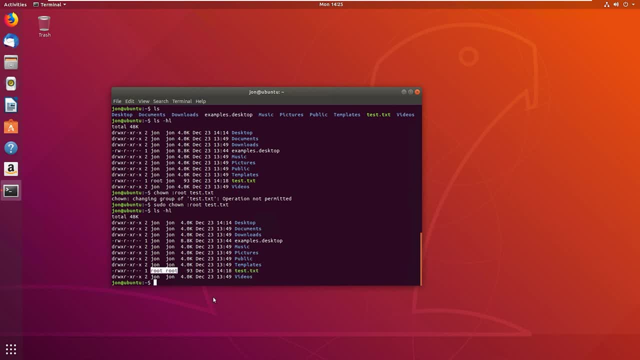 This used to be John John, Now it's root root. okay, Now if we want to change the user and the group ownership at the same time, we can change it back to us, And so we do the user colon, the group. 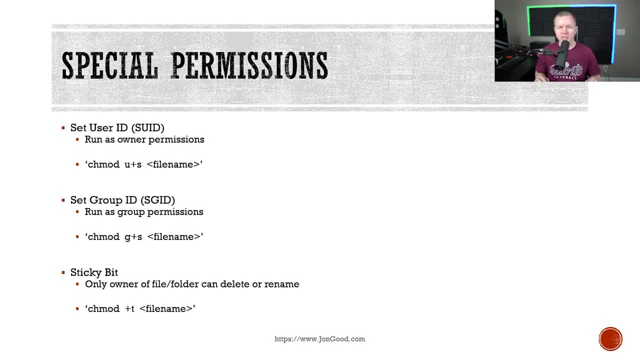 And if we look at that, Now let's change back to John John john, then we do the user colon, the group. Now let's change back to John John. there are special permissions within the Linux and Unix operating system that you're going to. 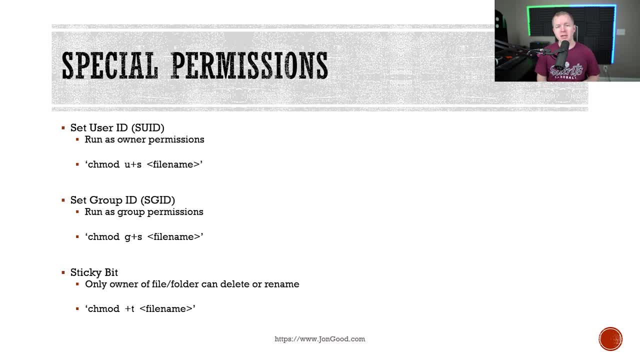 want to be aware of. The first is the SUID. Now, the thing with this is, if this is set on a file, and let's say it's an executable, whatever that script does or that file does, whoever can run it runs it at the permission level of that user. 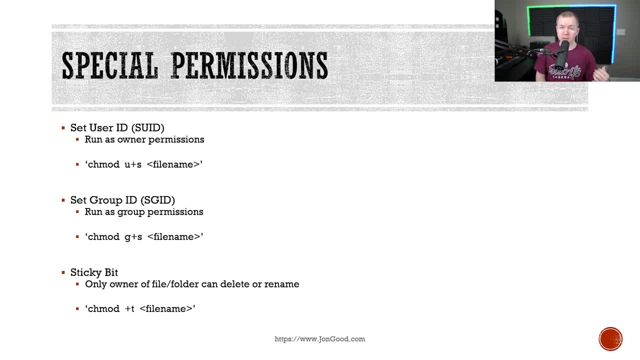 So like we were changing that file to the root owner, if that was a script and let's say it had add user in it- it was adding users- then if I can run that, I can actually run that as root and add users. That's very, very dangerous And these all kind of fall within that. 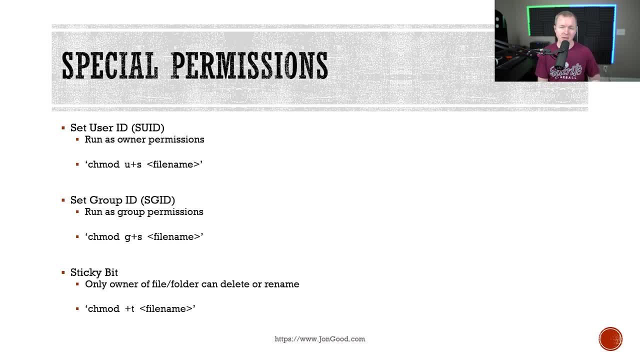 line, because you also have set group ID which does the same thing, except it uses the group permissions. Now if you see these in your environment, you want to be very skeptical if you're in security or IT or anything like that- because that can definitely pose a risk. 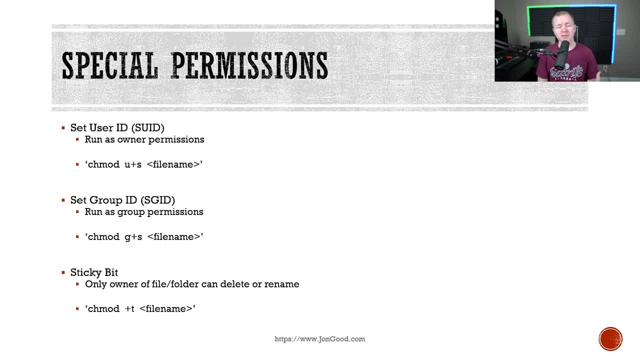 We then have the sticky bit which only allows the owner of the file or folder to delete or re-enter. Okay, So if you had a folder and you had information in there and the sticky bit was set, then somebody is not going to be able to actually delete things in there. 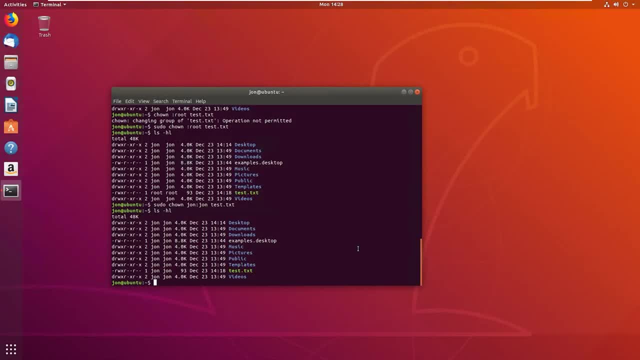 Now I want to show you what that looks like, just so you can see the permissions. We are going to set the user ID on that testtxt file. first We're going to do chamod, And actually I'll probably have to do this with sudo. So sudo, chamod. 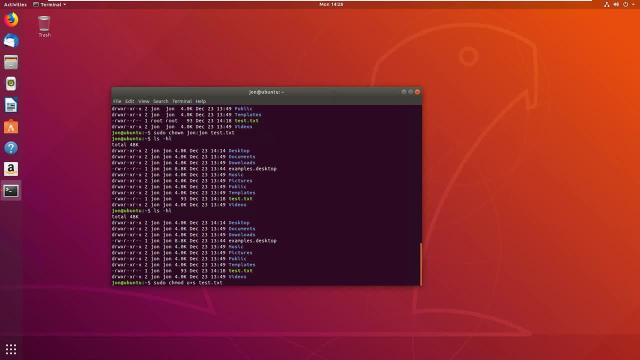 g plus s and then testtxt. Right, Let's look at what it shows. So, as you can see now it's red, so it's got a different color to it. Look in the owner column, here We have an s. 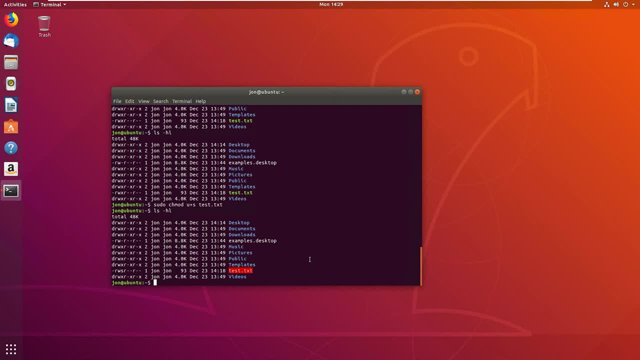 Okay, That is the set UID. Now, if we do the same thing, oops, sudo chamod g plus s and then testtxt. Okay, Let's look at the permissions. So now you have this s in the group section. Okay, So s s set UID, set GID. 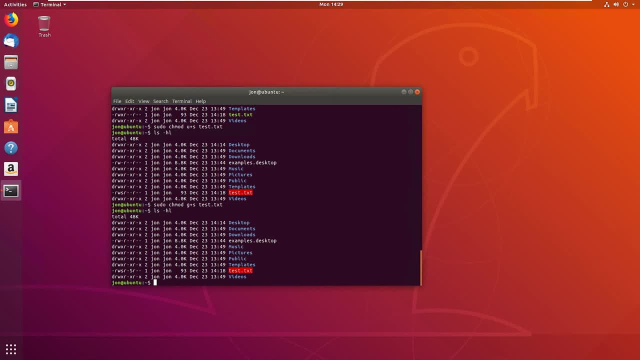 Now, if we're going to set the sticky bit, we'll do sudo chamod plus t testtxt. Okay, Let's look at the permissions. Now you have the sticky bit set, Okay, So if you see an s, an s or a t, be very alert, Okay. 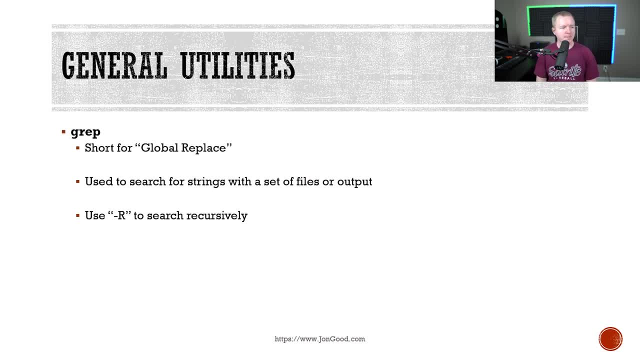 So let's go over some general utilities real quick here Now. we kind of already used this earlier on, but you have grep. Grep is short for global replace and essentially it is a search tool. Okay, So you can search through files. 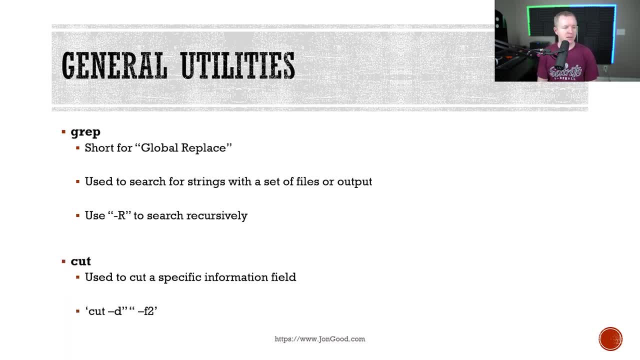 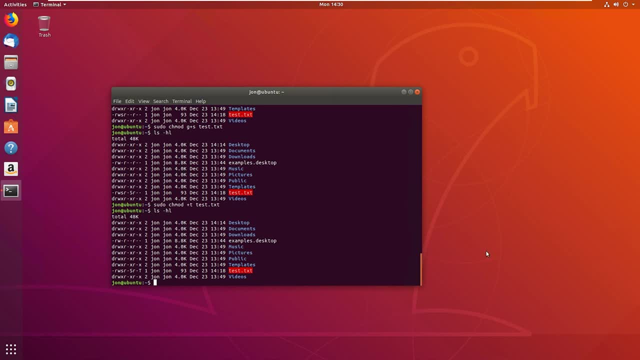 You can search through output- all kinds of good stuff. You also have the cut function or the cut command. I want to show you this real quick so you can see this. Let's do an ls here. Okay, So we'll use the testtxt again here. 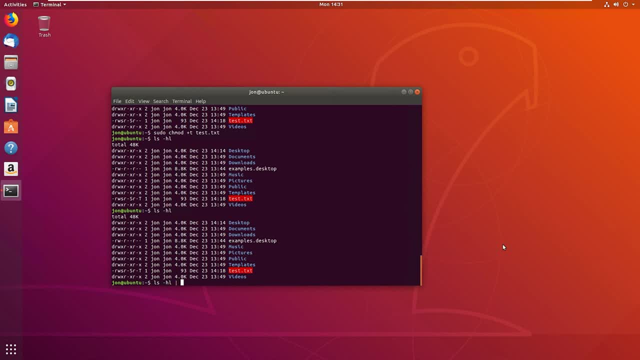 So we're going to list everything in this directory, We are going to grep, we're going to search for testtxt, Okay, So that will give us just that information, And then we are going to cut a specific field out. Okay, So with cut, you have. 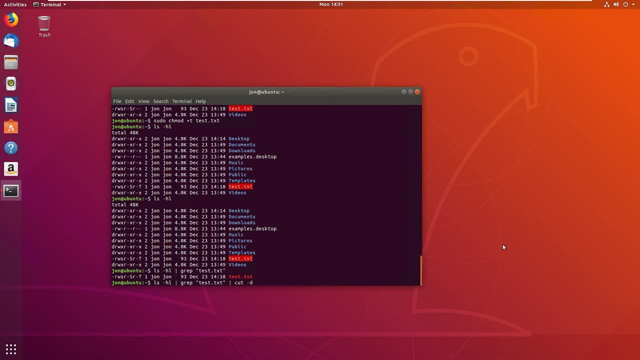 the cut dash d, which stands for delimiter, You have to provide what it's going to cut based on. So we're going to use spacing, So we'll do quotes here with a space in between, and then you provide the field. Okay, So the number. 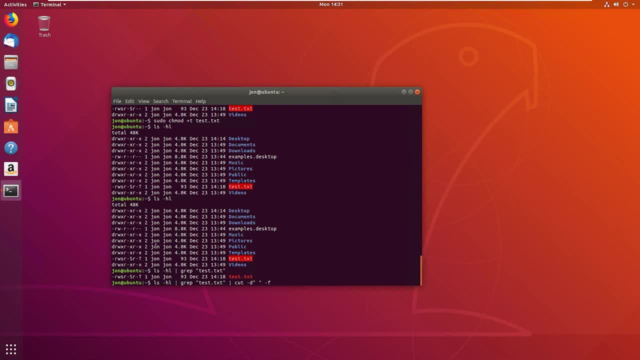 that you want it to cut. So one, two, three, four and so on and so forth, Okay, So we're going to do the field of two, Okay, And that gives us a one. So if you look up here, 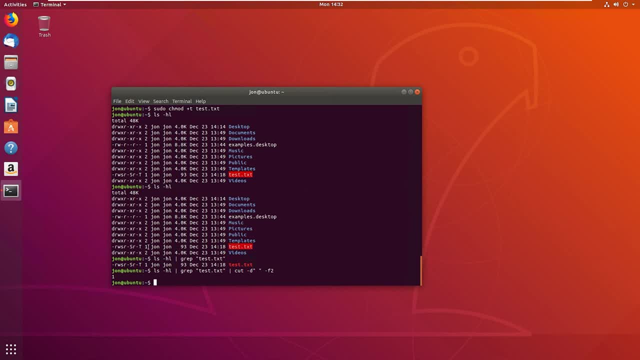 where is that one? That one is right here. Okay, That's the second field. So then, if we do three, four, let's do five, And hopefully it might. we'll have to see what it gives us, but hopefully it gives us this. 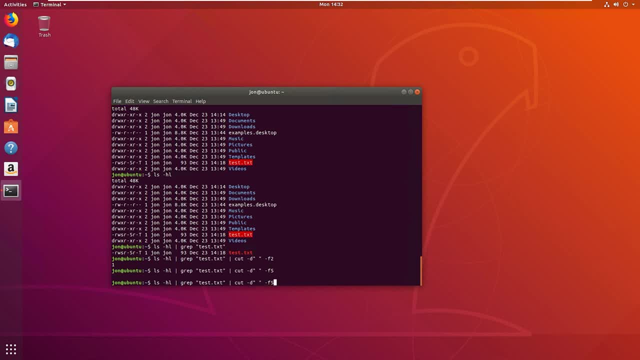 So let's change that to a five, Okay, So that there's an extra space in there. Six, Nope, Seven, Okay, So just because there's some extra spaces in here, but seventh field is right here And so you can do that for whatever you want. So if we do eight, eight is actually going to give us this field here. 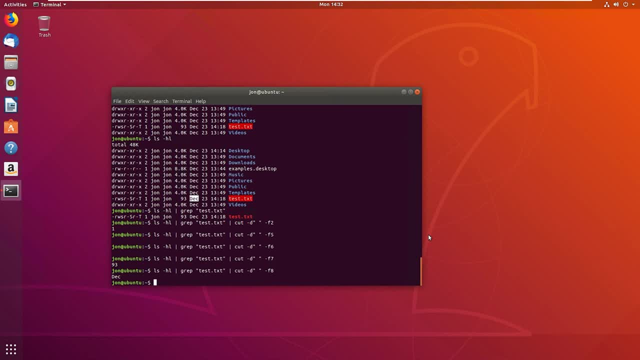 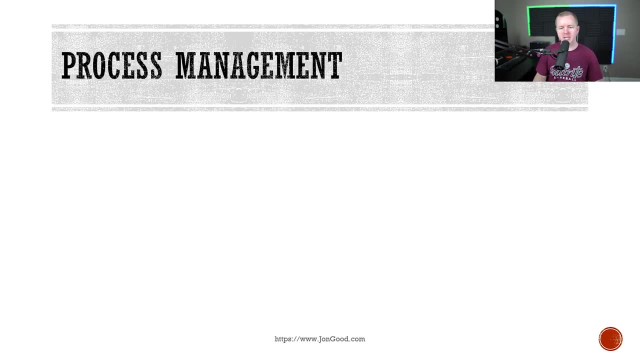 Let's do that, We go. So the cut can be very useful to cut out certain types of information. Now process management. process management is a little bit different on Linux and Unix than it is in windows. Some of the commands You're going to want to know, our P, S, P? S can show you the current running processes on the system. 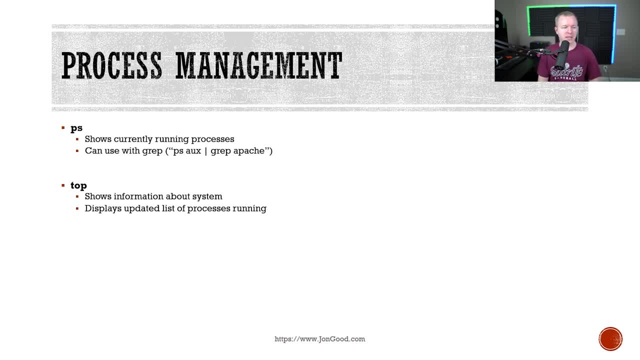 The top command is going to show you the top running commands, So it sorts them. the kill command That's if you want to kill a specific process and then you have kill all where you can actually kill based on a certain name, everything associated to that. 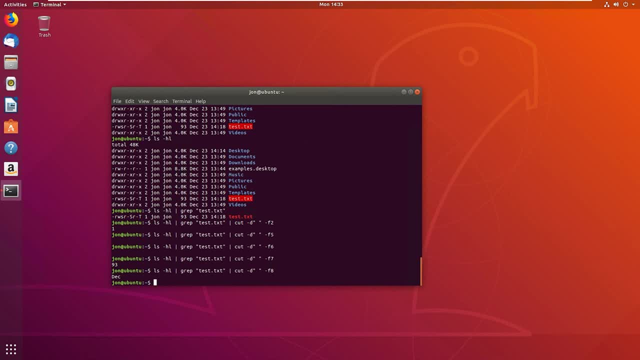 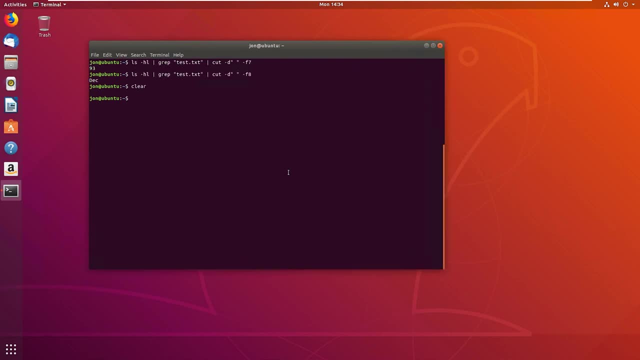 So let's go over to the demo page here To show you- let's actually clear this out here and make this a little bit bigger. So we're going to do the P S command So you can see a few of the commands that are running. a command that you would want to run on here would be P S. 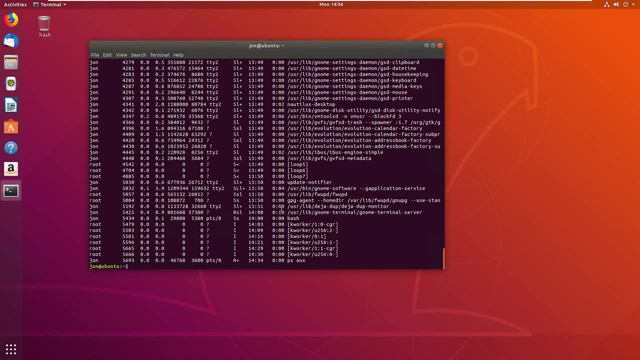 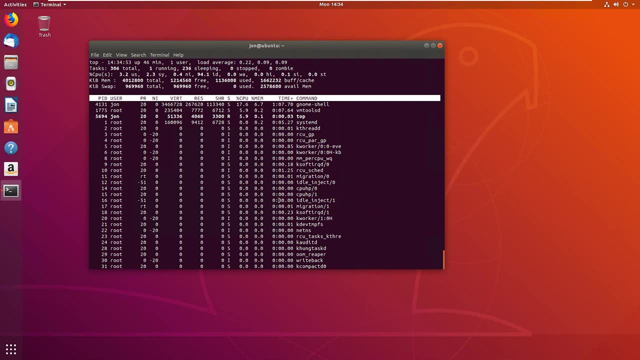 ogs And you'll get a whole bunch of different processes that you can see on here. If we do top Again, that sorts all the different processes that are running. It gives you a little bit more information about what's going on. The user running it. P I D. 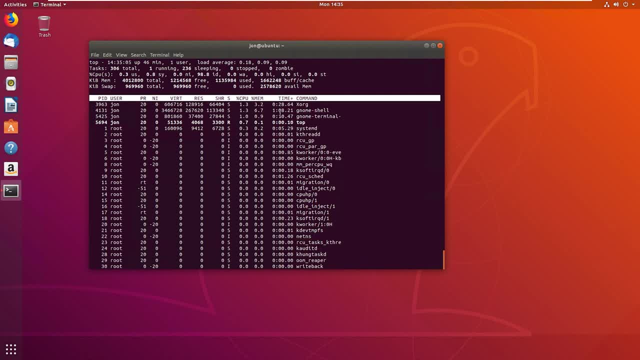 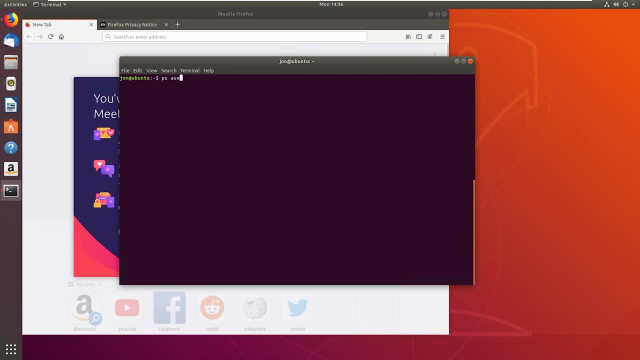 which is the process I D, And then I just hit Q to quit out of that. So if we want to kill an actual process, let's go back in here and let's search for Firefox, which I just opened up, Right, And so this is the process I D that we want to kill. 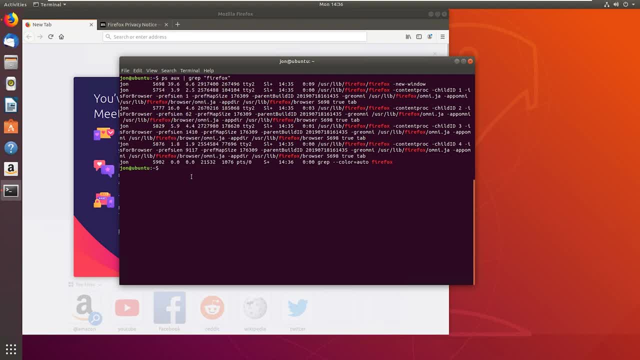 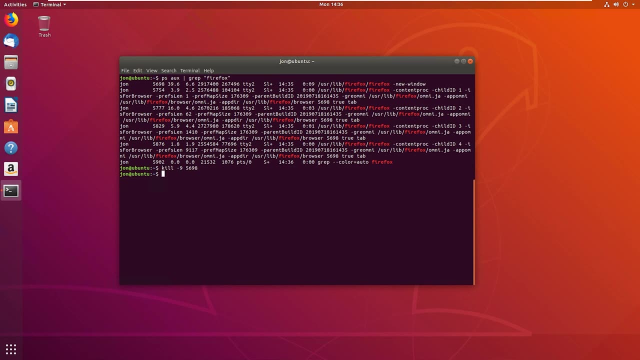 So we're going to Copy That And we're going to do kill And it a signal- nine is what it's called- and paste that in there And then you can see it killed that Firefox process. Okay, Super easy, super useful. 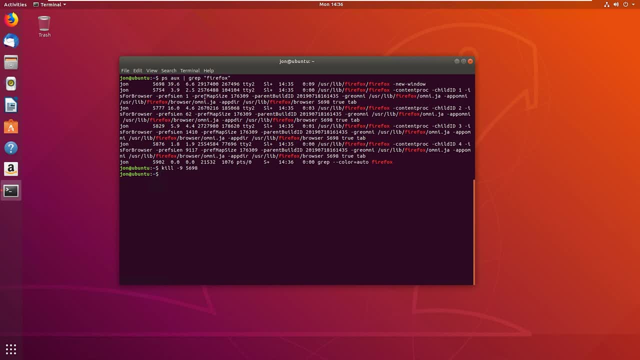 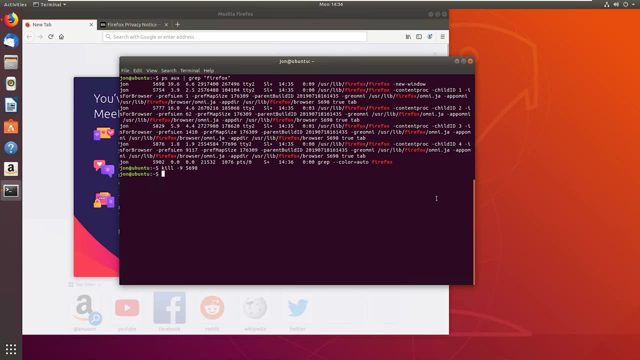 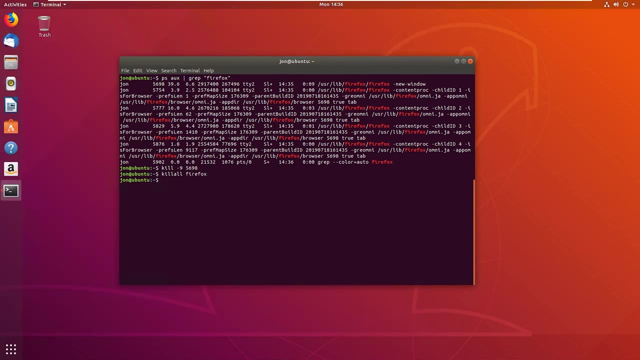 And then, if we want to use the kill all command instead of that, let's open that back up here and we'll use: Use the kill all. and then Firefox- Same idea- Kills it all. Now, that's useful if you have a bunch of child processes especially. 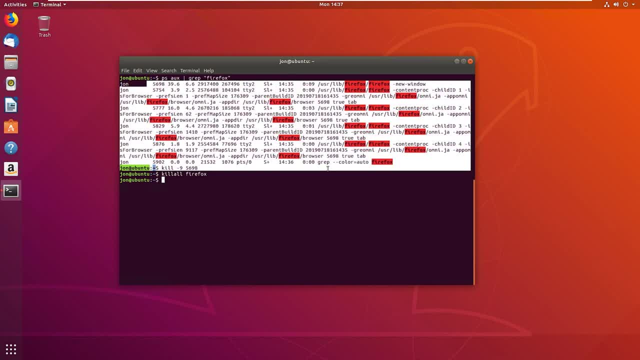 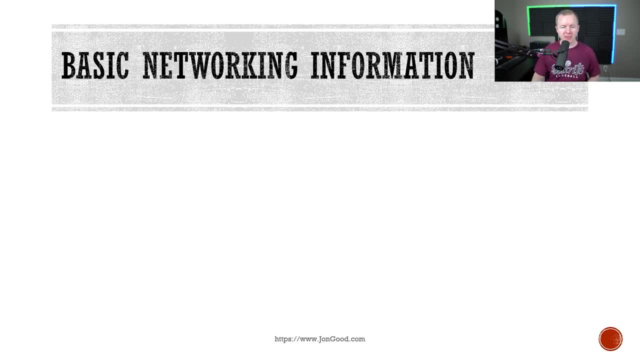 So, like with Firefox, you can see it open to all that stuff which, more than likely, it killed out. but kill all. we'll just kill everything that's labeled Firefox, a basic networking information that you're going to want to know for Linux. 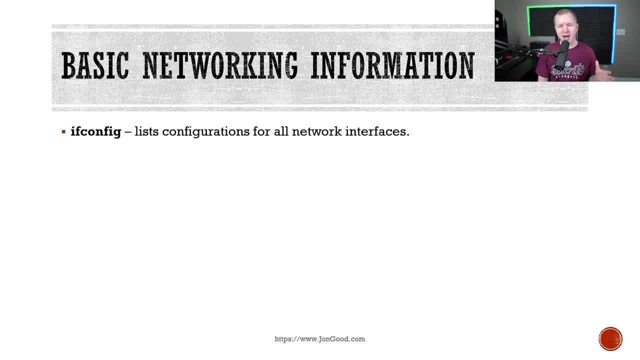 You have. I have config similar to windows. You had IP config. This is going to list all the network interfaces of net stat. That's going to show a bunch of information about network statistics, routing tables, services, running things like that. 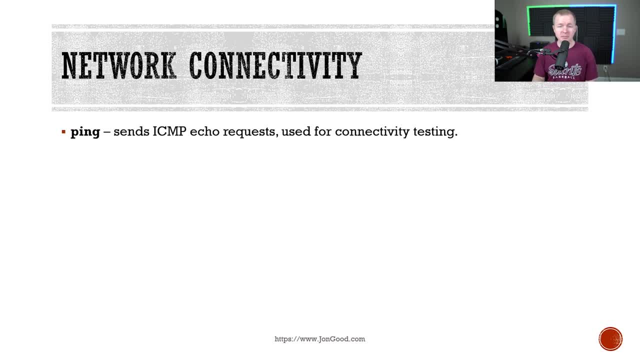 There were connectivity. You have the ping command, pretty standard across different operating systems: sending out ping packets, ICMP packets, test connectivity trace route. trace route will identify the path that a system is taking to send It's data to a destination. 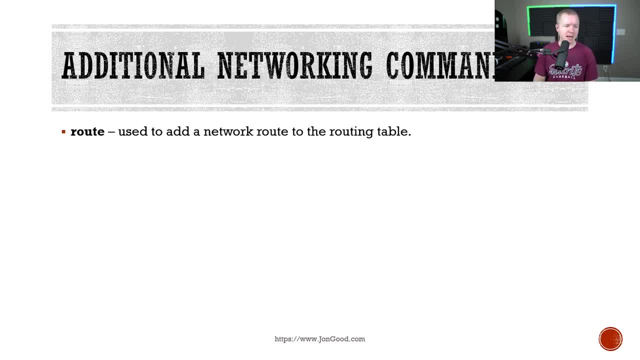 And then a few other additional commands. You have the route command. You want to add a network route to the routing table. You have the art command. shows the store art entries or the Mac entries in the art table. Now let's get into software management here. 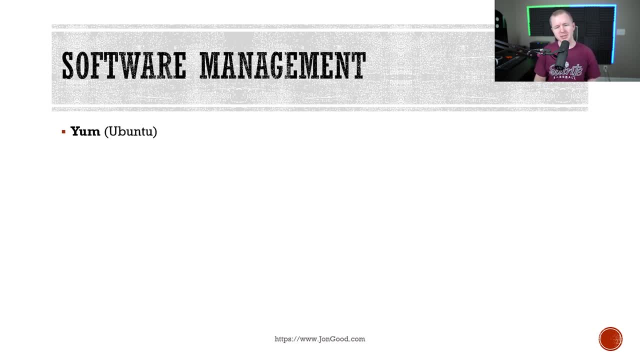 So, depending on the operating system that you have, you have a few different package managers. for Ubuntu, You have yum And to install a package you have yum. install the application, You can update it by doing yum, update the package and then remove the package by doing yum. 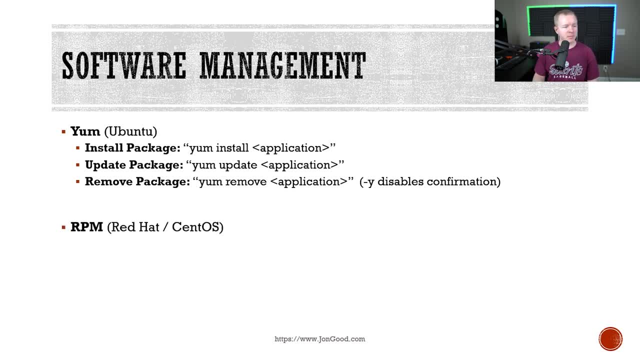 Remove the application or the package. RPM is the other style. This is what you're going to see on Red Hat and CentOS. Basically, it's the same idea: RPM dash I to add an application. RPM dash capital U to update that application. 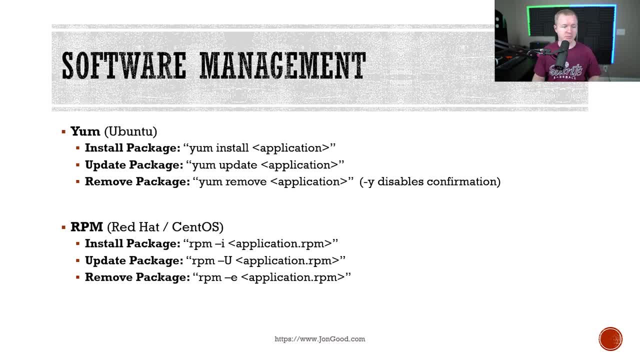 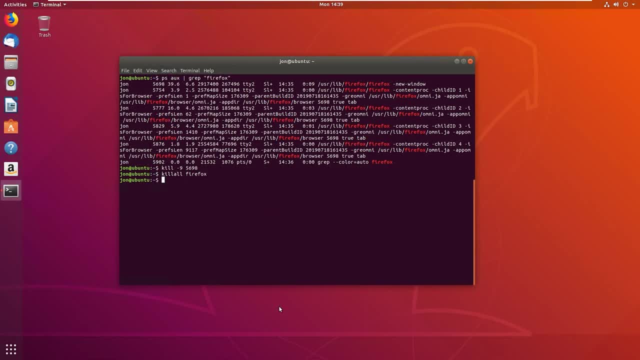 And then RPM dash E To update that application. If you wanted to remove that application, let's go and show you here on the Ubuntu box here. So we're going to do yum install and let's just do terminator. Okay, so I do not have yum installed right now, so I'm going to install it real quick. 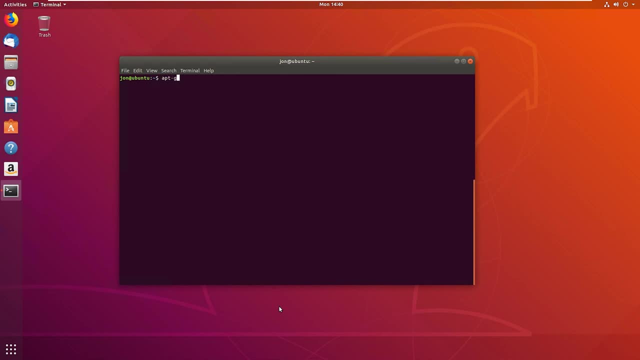 And then I forgot to mention was the app git, which you can do: app-git install and we'll just do my SQL And it's going to make us actually be root user. But if we do it like that, then it would just go through and install it. 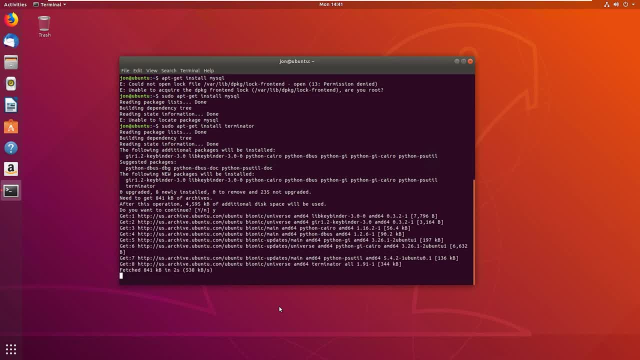 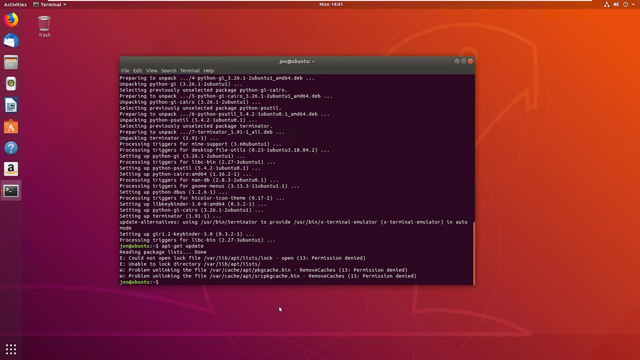 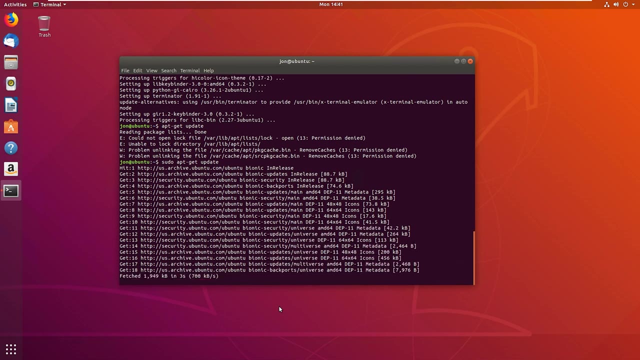 There we go, And with that you can actually do the same way. So app-git update, Sudo, app-git update, And it just goes through and updates everything. If we wanted to use yum, which we installed, we didn't really have to install it. 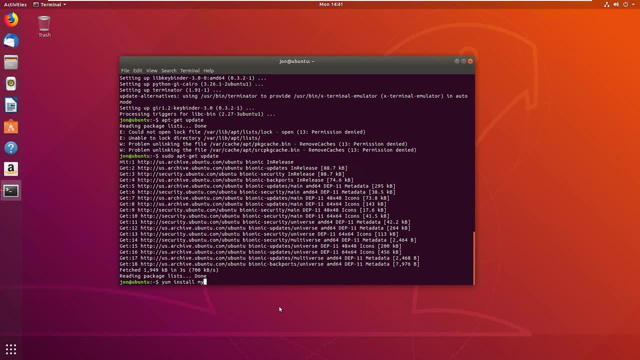 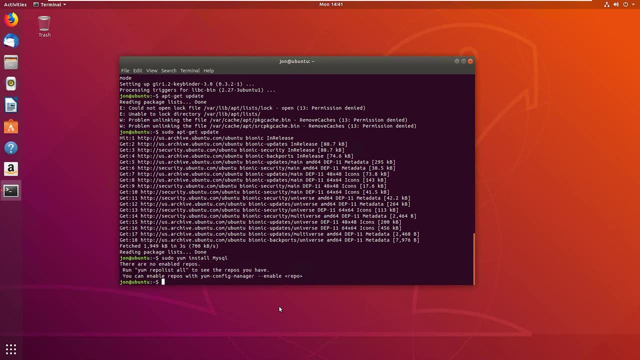 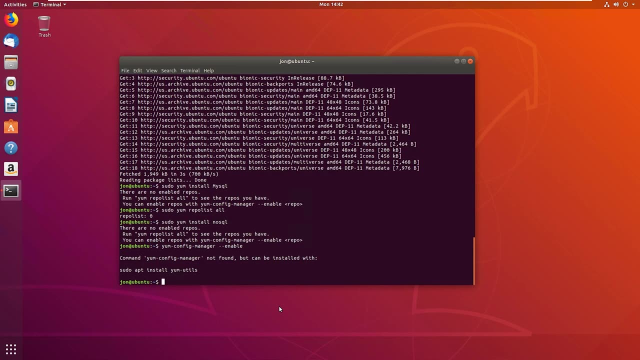 But yum install and let's- actually we'll probably have to do sudo for this- Yum install my SQL, Let's see if we can get it on there. Let's see here. And apparently with yum there's a lot of different configuration things that you have to actually configure now. 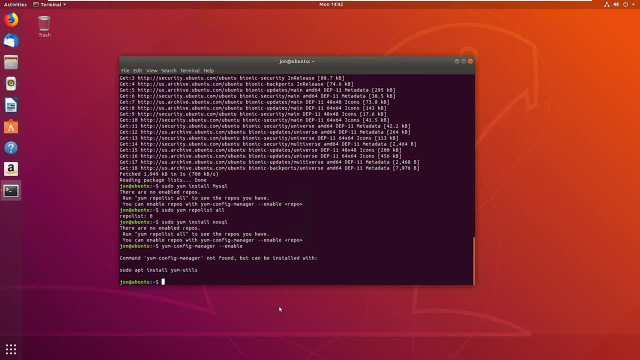 But either way, you can go through and install the yum and set it all up, Or you can just use the app-git. That's what I tend to use now is app-git instead. It's a little bit easier, Especially when it just comes with it. 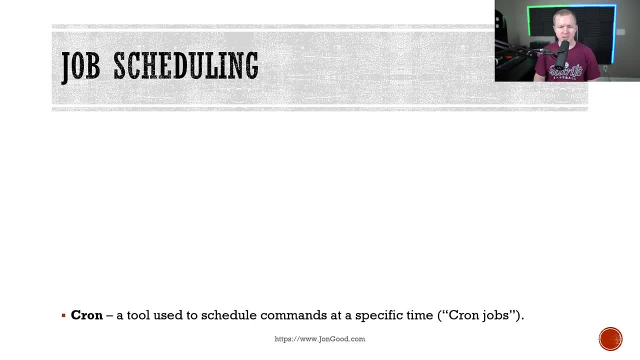 All right. so job scheduling: I don't want to get too in-depth into this because it's kind of more of a complex thing, But with job scheduling in Linux you use something called a cron job And this is to schedule a certain task at a certain time. 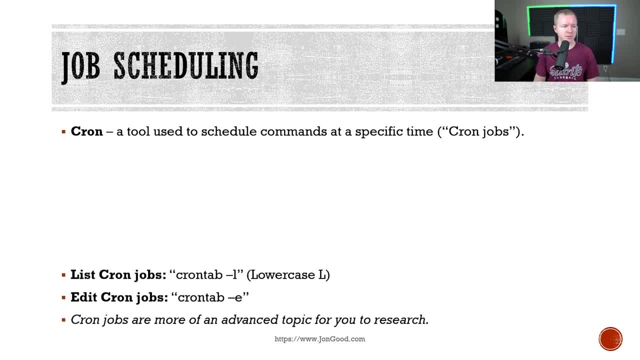 You can set it up to run frequently one time, anything you want to do. If you want to list the different cron jobs that you have, you can do cron-tab-l, And if you want to edit them, you can do cron-tab-l. 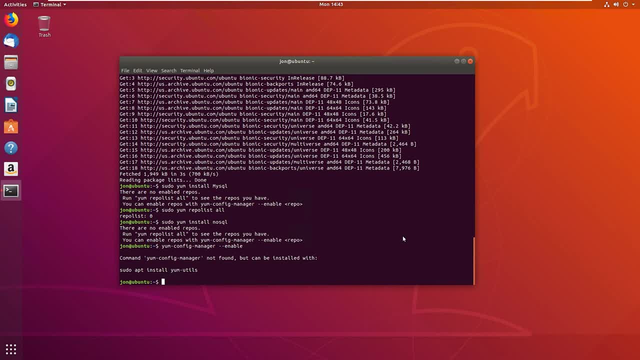 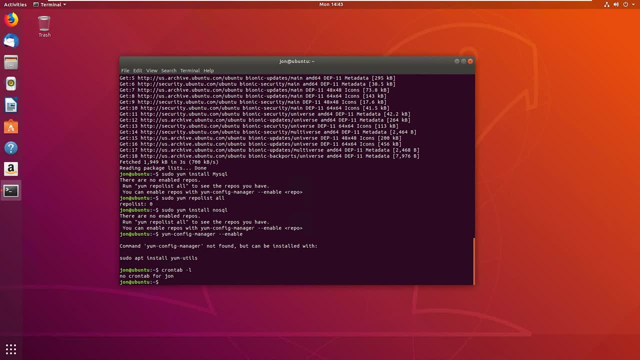 So I will show you that real quick here, just so you can see what it looks like, But cron-tab-l to list them. So I don't have any cron jobs set up yet, But it would show it in there, Cron-tab-e. 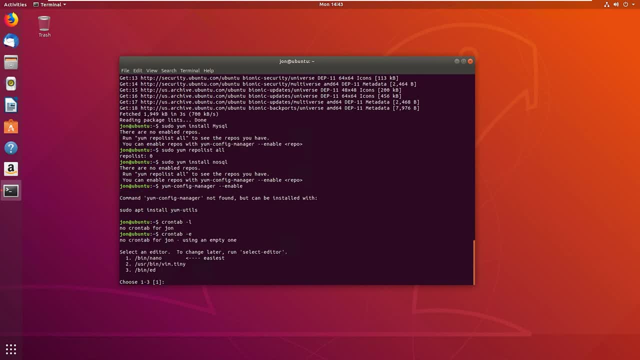 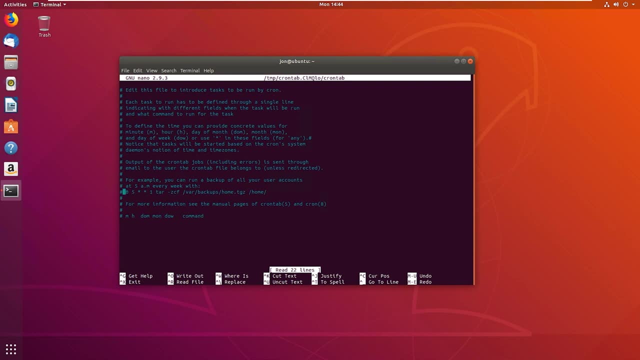 And then you can actually set it up in here to edit, And that's it. So again, this is a sample command right here, But I'm going to leave that up to you to research a little bit more if you want to set up different jobs. 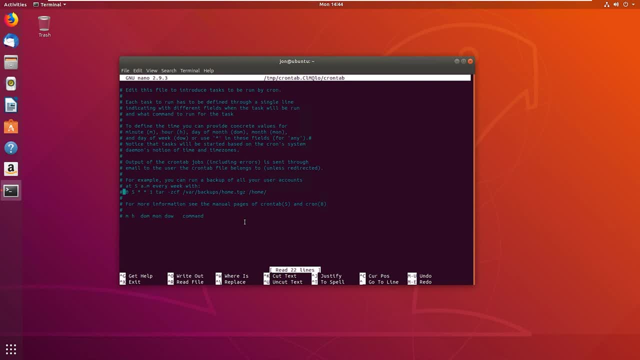 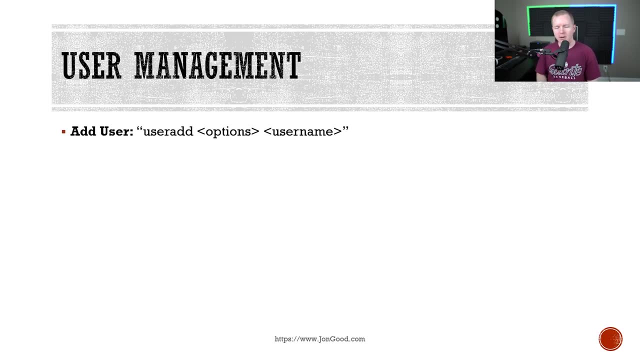 Because, again, it's a little bit more complex than just kind of the entry basics to the Linux operating system. All right, So let's talk about user management Now. if you wanted to add a user in the Linux operating system, it's very simple. 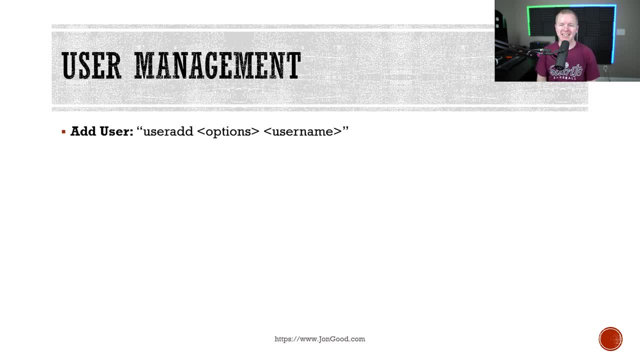 You go to the command line and you can do user add any options that you want to do and then the username. There's a whole bunch of different options. You also can modify that user once you've already created them. So you can do user mod again any options that you want to do and then the username. 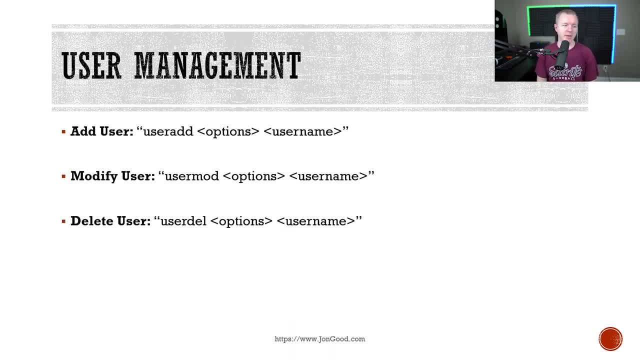 You want to delete a user- user del- and then any options and then the username. Super easy. If you want to set the password for a user, you can do password and then the username. It will then ask you for the password that you want to set. 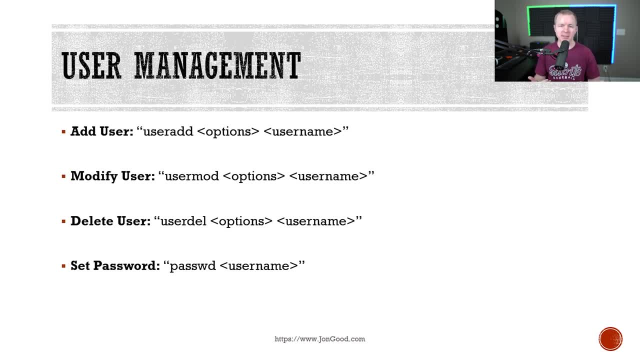 Instead of entering the password in where it's going to be clear text. it would then just basically hide the password that you're typing in, so it's never shown on the screen. And then, if you want to view or modify password expirations, you can use the age and options and then the username. 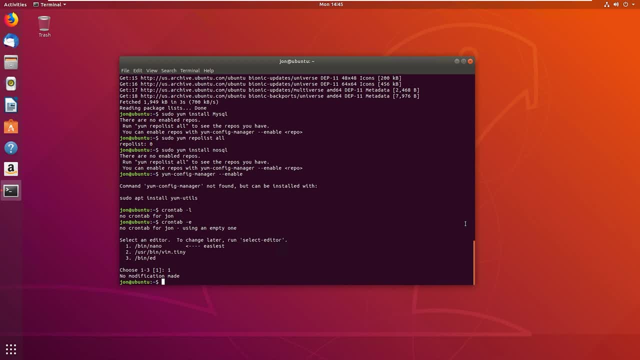 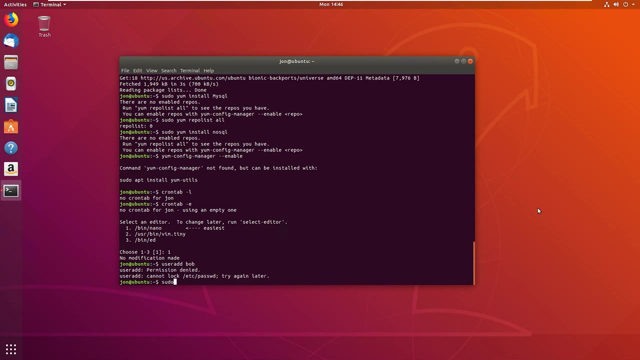 So let's go to the system here and we'll create a user here real quick, just to show you. So we're going to. We're going to do user add. we're not going to do any options, we're just going to use the default. we're going to add Bob and I need to actually be admin, so I need to run this as root. so we added the user Bob. so now you want to set the password for Bob. 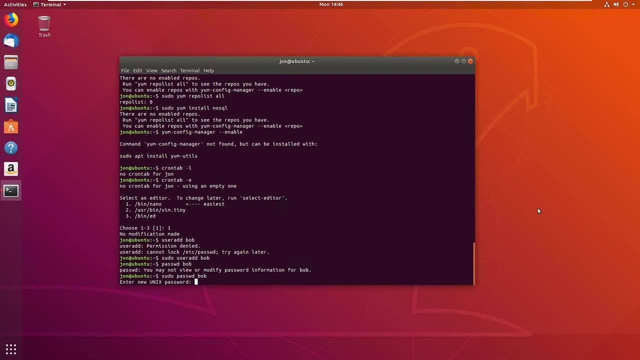 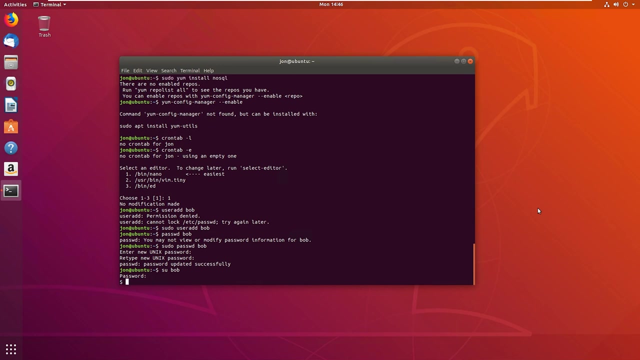 There we go. so let's enter his new password: 1,, 2,, 3,, 4,, 5,, 6,. okay, 1,, 2,, 3,, 4,, 5,, 6, and Bob's password is now 1,, 2,, 3,, 4,, 5,, 6,. so now, okay, if I switch user, so SU, I'm going to switch to Bob and I'm going to enter 1,, 2,, 3,, 4,, 5,, 6,. okay, who am I? 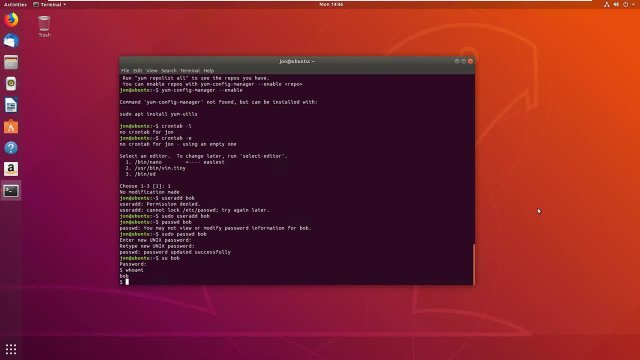 I am Bob. Okay, and then that's how you can switch between different usernames. So I will type exit and that will exit me back to being John. Now, if I want to delete that user- sudo, user del- no options and we're going to delete Bob. 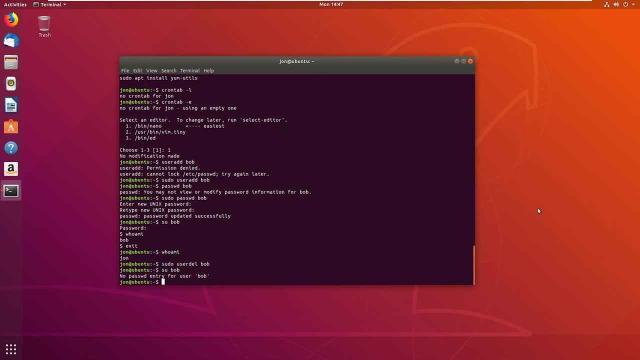 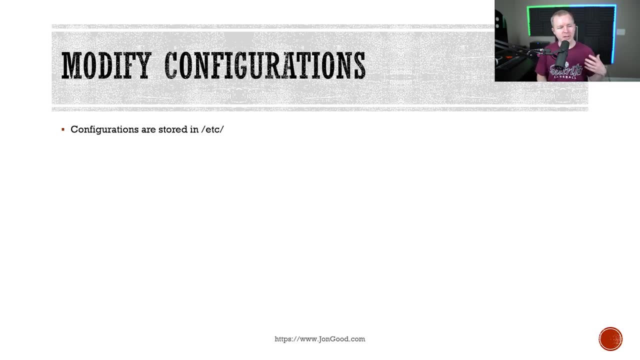 And now, if we try to switch to Bob, no password entry for Bob. Bob has been wiped off the system Modifying configurations. So, like I said, all the configurations are stored in the Etsy folder. You can actually modify these configuration files with VI, which is the standard configuration editor or text editor in Linux. 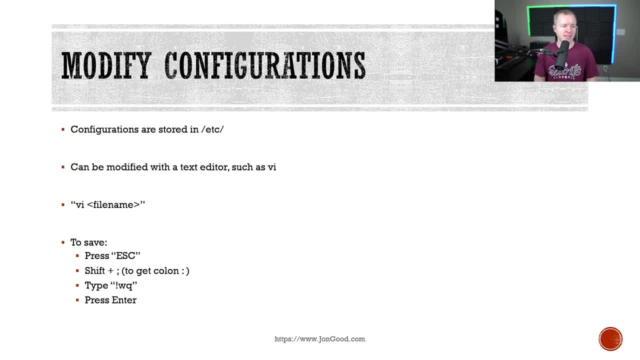 You would do VI and then the file name, and that's how you would get into it. Once you are ready to save a file- so you've modified it- you press escape, then you do colon, so shift, and then the semicolon. 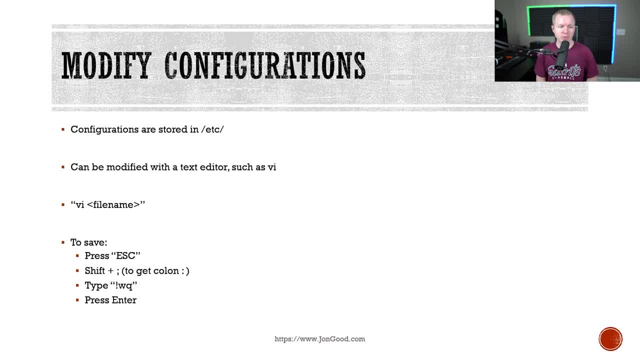 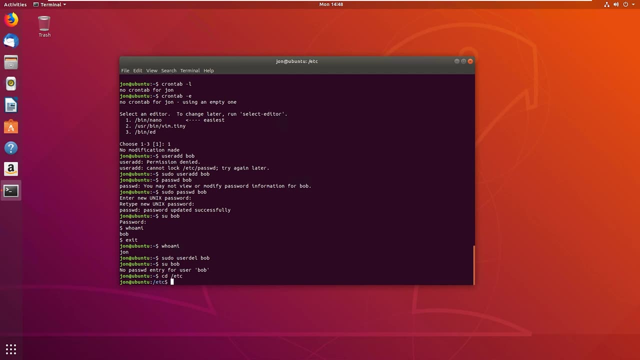 And you type exclamation WQ and that writes and then quits and it forces it to be written to okay And then you press enter. Let's go to the system. so I can just show you that real quick If I go to the Etsy folder. okay, let's list out what's in here. 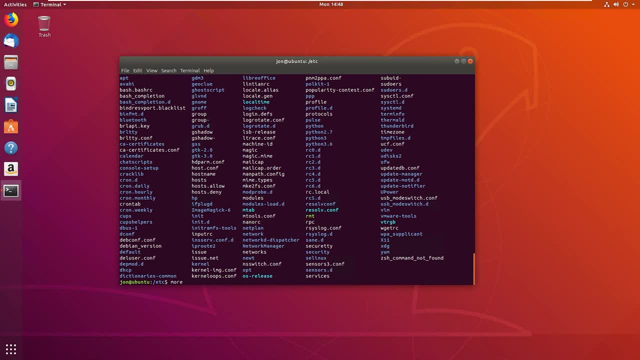 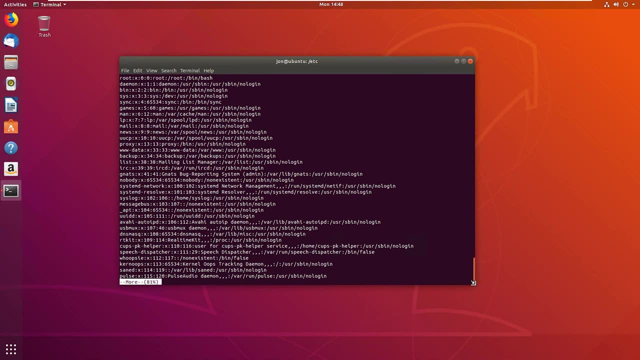 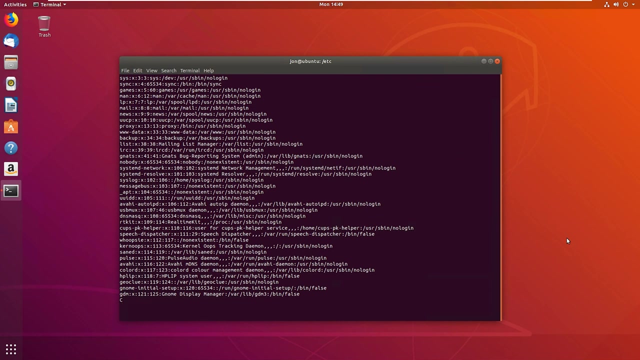 And let's go ahead and look at the password file. Okay, so this is where all the user information is stored. If I want to edit some information in that file, go to the end here And I can type whatever I want: Press escape, press shift and then semicolon to get a colon. 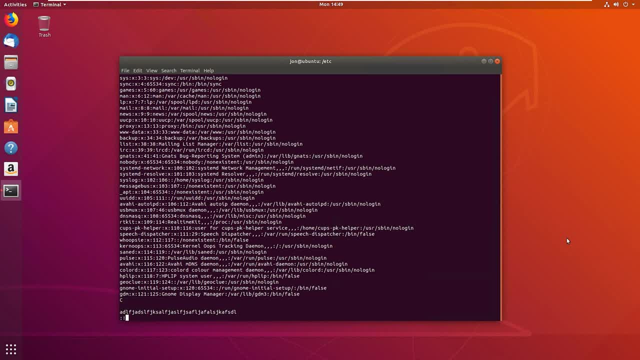 You can see that it goes to this colon. You type exclamation, right quit. So I'm not actually going to do that because I don't want to save this, but that would force that file to be saved. okay, Now, same thing. if you just want to quit out, sometimes you'll get a notification that read-only, or something's changed or whatever. 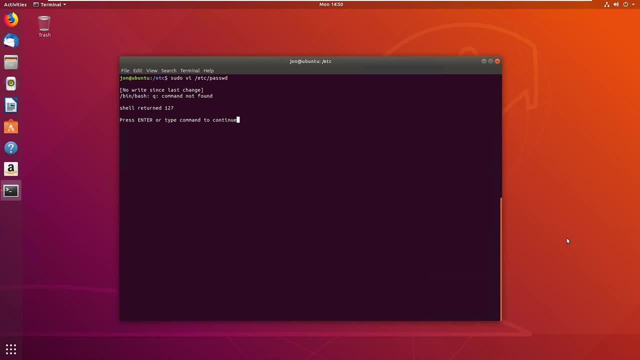 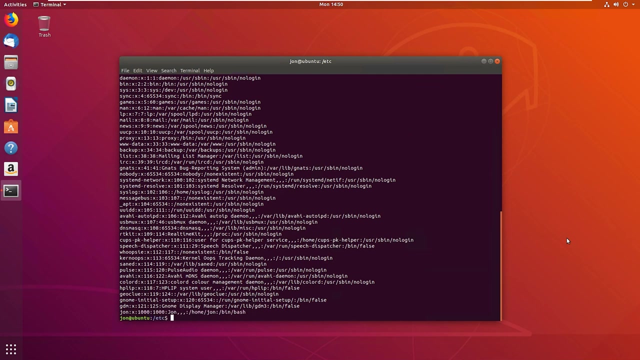 You do exclamation and then quit, It is not going to save that information. Okay, and then if I go ahead and go back into that file, it has not saved that information in there. All right, let's talk about reading logs now. 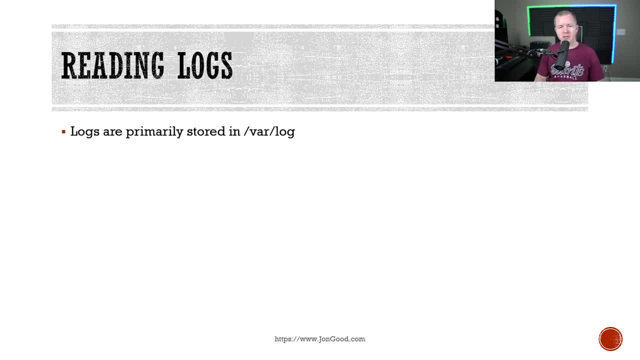 So logs are primarily stored in the slash- var- slash log folder location. You can read the logs using cat, more or less of those commands. If you want to keep reading a log file, you can do the command, You can do the command, tail, dash F and then the file name. 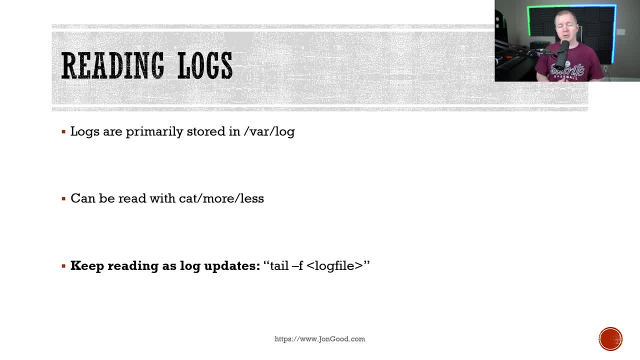 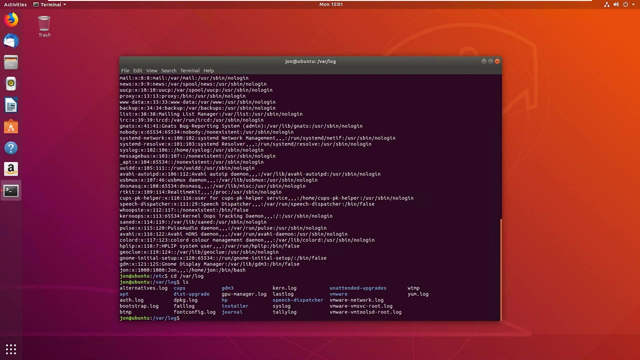 You can do this really with any file, but it's really useful for log files because it will constantly keep updating that information. Let's go over to the system here. So we'll go to the location for the log files And these are the different log files that you have. 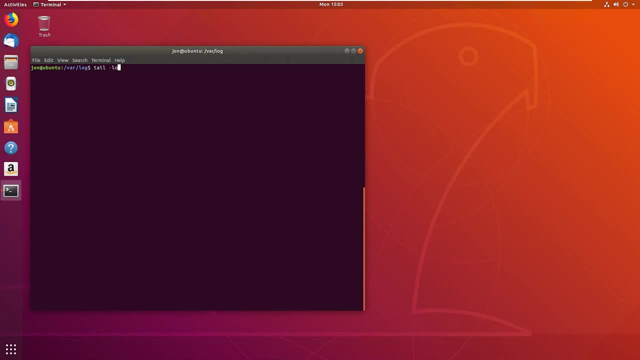 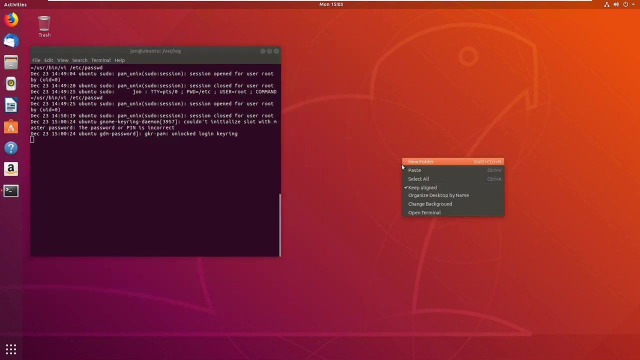 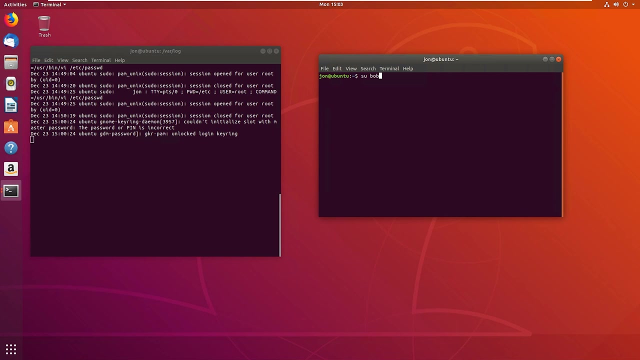 So let's do this on the auth log file. Okay, so keep in mind the bottom one. here is a wrap, The unlocked login key ring. So open up another one and we'll generate some events. So, as you can see here, try to log in. try to switch to Bob. 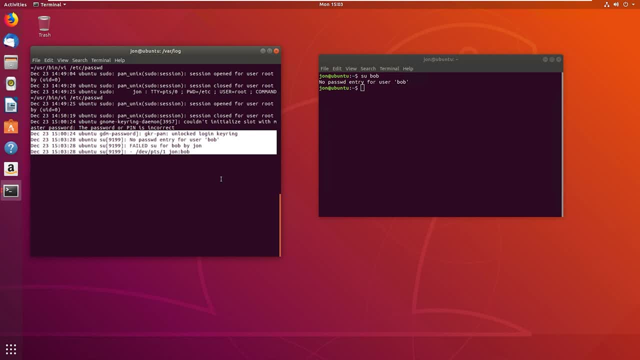 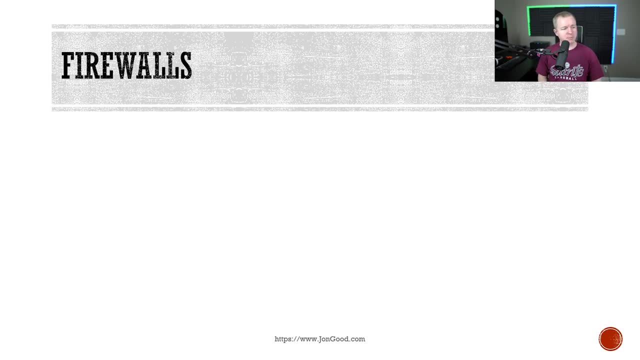 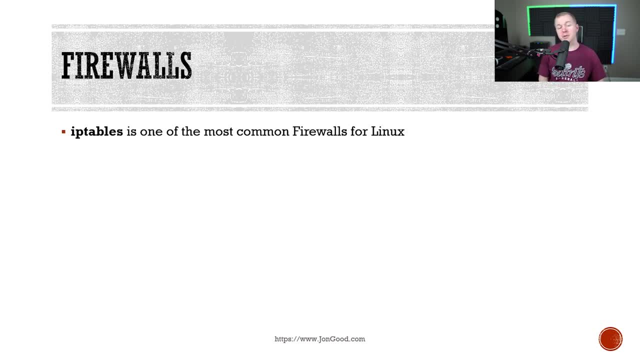 So IP tables is one of the most common firewalls used on Linux. If you want to list the rules, you can do IP tables dash capital L. You can also add rules, Just like any firewall. you can decide to drop traffic from certain networks or IP addresses or allow it. 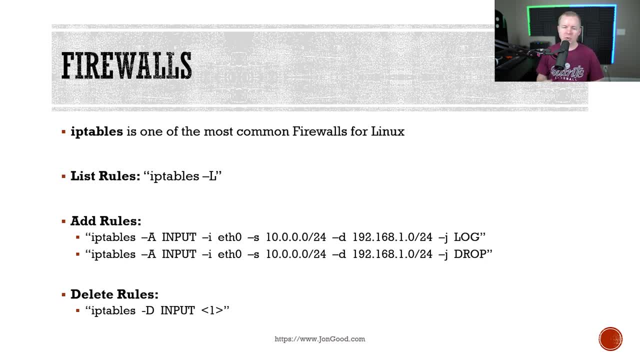 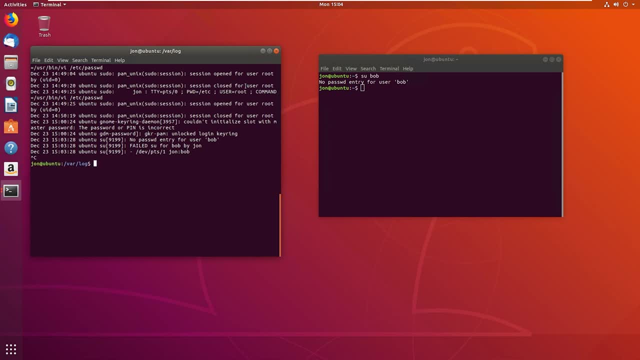 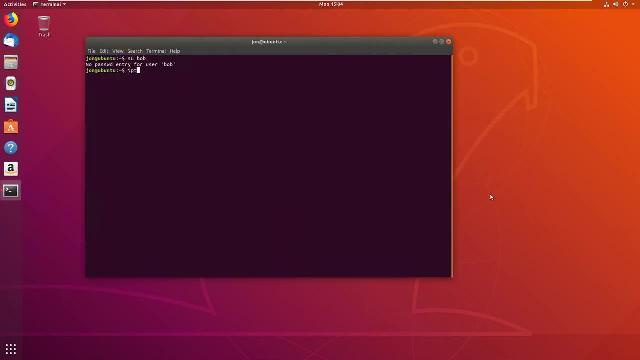 And then you can also delete or remove those rules. So let's go over to the system again here And we'll close this out. So let's see if we have any rules that are configured, And it looks like I need to install IP tables. 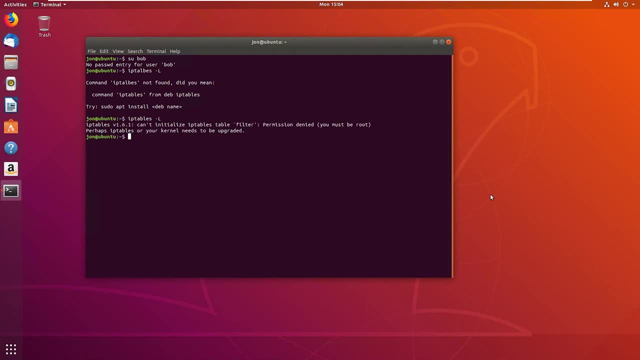 Actually I didn't even spell it right, So you have to be root. So tables dash L And then my password. Okay, so there are currently no rules configured, So let's add a couple rules. So we're going to do IP tables dash A. 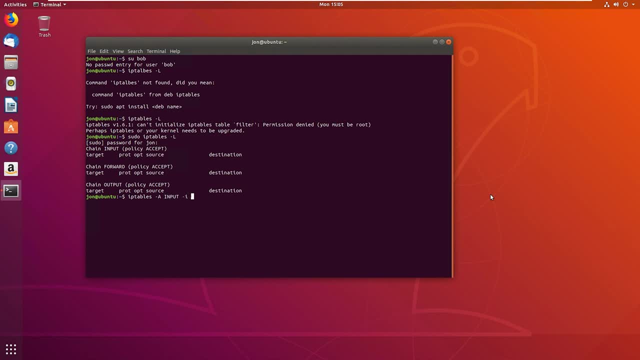 We're going to call this input, We're going to put in the interface of zero The source And 0.0.0.0 slash 24, destination, 192.168.1.0.. And it doesn't even matter if these are ours or not. 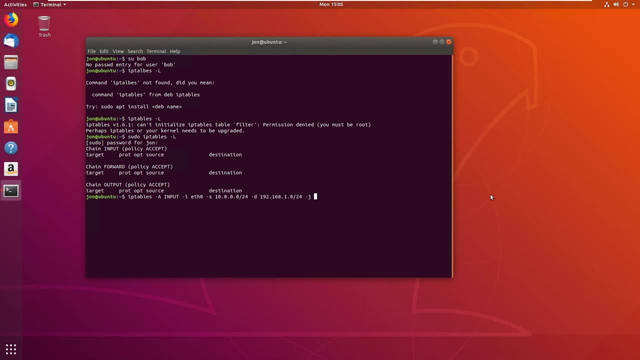 We're doing this just for representation purposes And we're going to log that information And I've got to be root to do it. So sudo, Here we go, And we're going to add one more here. So sudo IP table. 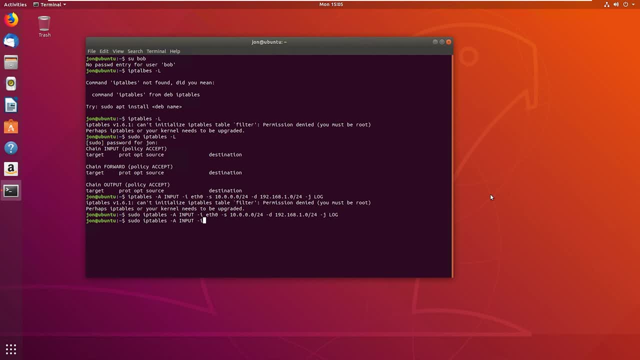 So we're going to do IP tables. dash A, Call it input. The interface is the same interface, The source is going to be the same And we'll put our destination here And we're going to drop these, Okay. So now let's do sudo IP tables.